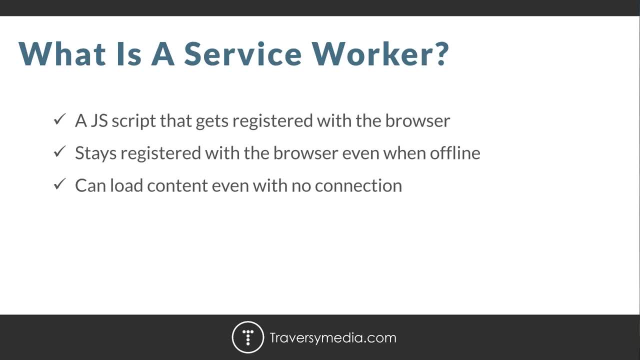 or your application and their connection goes out, they're still going to be able to get that information, And this is a huge requirement of progressive web apps, because it makes it seem more like a native app. Now, usually when you go to your browser, you enter a URL for a site: the 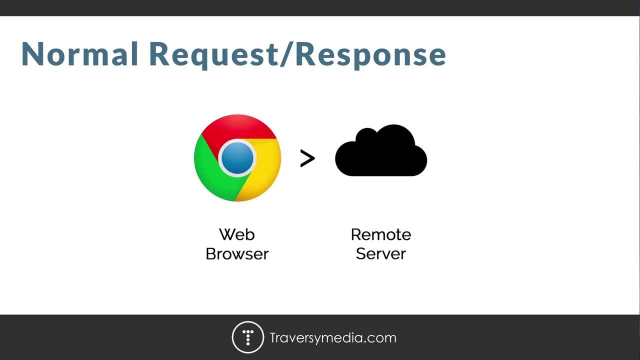 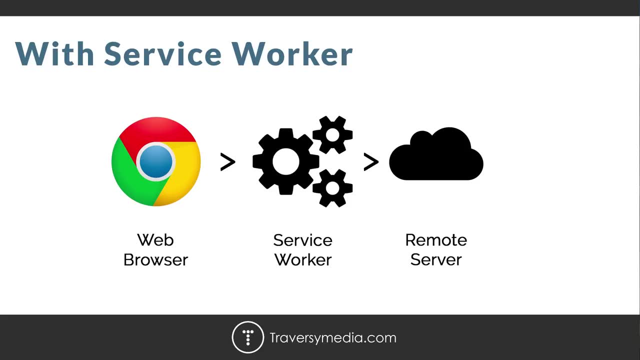 browser fetches it and the remote server returns that information to you. But when you have a service worker registered it basically adds another step to the process. The service worker kind of jumps in the middle And it can intercept the request and then decide what should happen. So it decides what can happen. 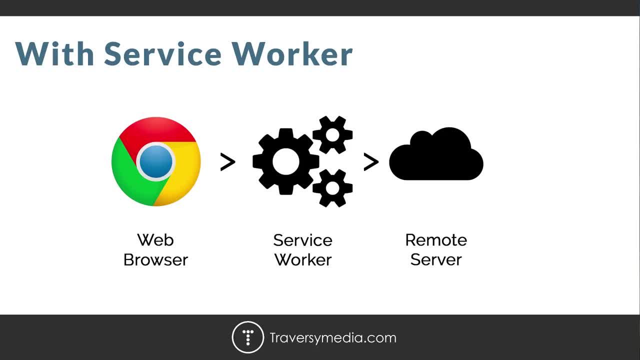 with that request in terms of showing the remote version or showing an offline version or whatever it is you want to do. And doing this can prevent that. really ugly not found, not the 404 pages, but the default browser page when your internet goes out, So you can even have custom offline. 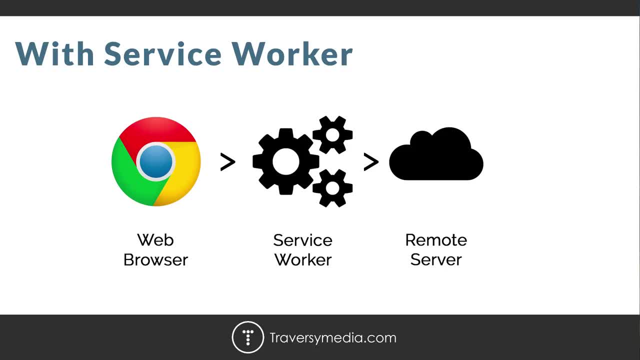 pages if you want. If you're not, you can't get that out. And that's pretty cool, All that stuff, but I don't know if you've ever seen a service worker registered with a browser and their You're not going to cache the entire site in general. 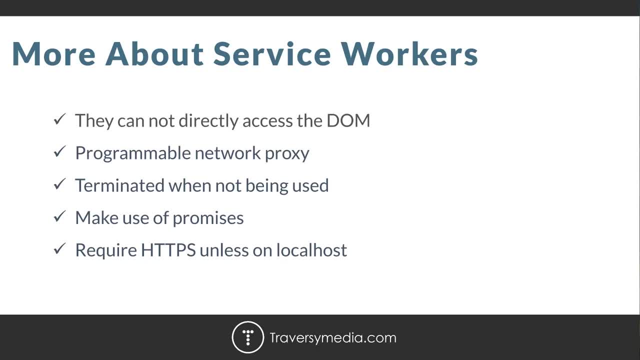 So some other facts about service workers. they can't directly access the DOM, the document object model. instead they communicate with the pages it controls by responding to messages sent by something called the post message interface, and those pages can then manipulate the DOM if needed, but it doesn't access it directly. 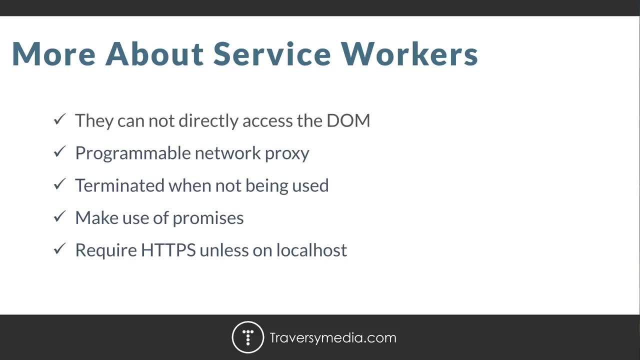 A service worker is a programmable network proxy that allows you to control how network requests from your page are handled. Service workers are terminated when they're not being used and then they're restarted when they're needed again. They also make use of ES6 promises, so you'll be seeing a lot of then catch and then. 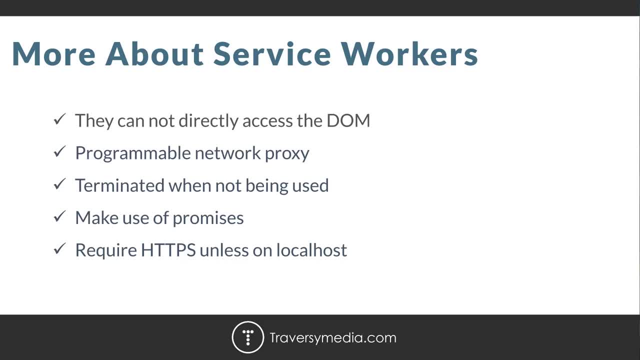 a really important part of service workers, or a really important piece of information to know, is that you need HTTP- HTTPS- unless you're on a local environment and you're using local host. So if you upload to a remote server, make sure that it has HTTPS installed and enabled. 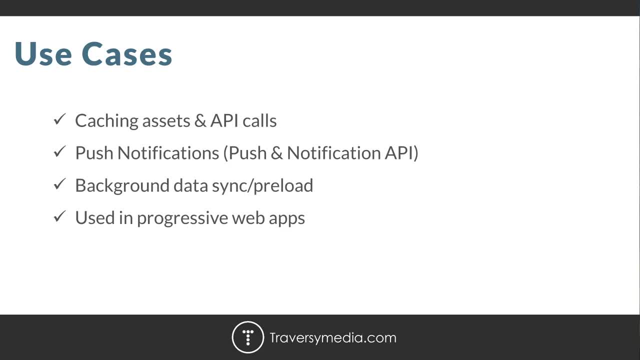 So most commonly, service workers are used for offline browsing and caching assets and API calls, but notifications are also a big part of service workers. Those are the little notifications that some websites have that'll pop up on your desktop or on your mobile device. 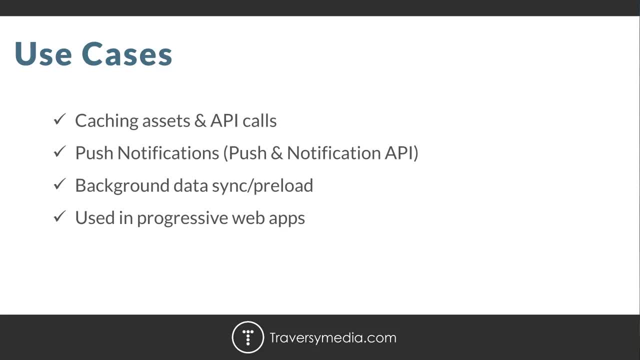 And they're really great for marketing and advertising and so on. And I did do a course on push notifications and Nodejs using service workers. I think it was about two months ago that I did it. If I remember, I'll put the link in the description. 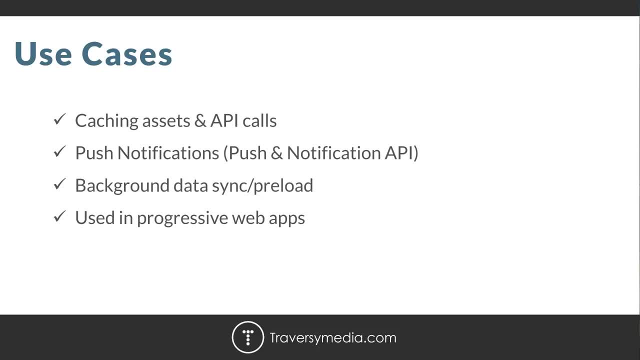 There's also something called Background Sync, which still isn't fully supported in all browsers, but this is a new API that lets you defer actions until the user has a stable connection. Okay, So if a user, for instance, likes a service worker, they can defer actions. 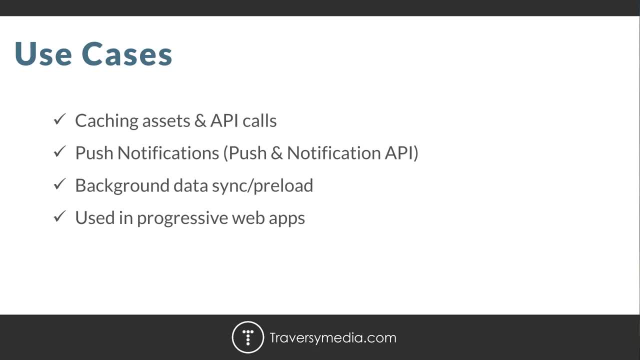 If a user, for instance, likes a post on a social network, this is a case where something needs to be sent to a server, which isn't possible without a connection. But with this browser sync API, it allows that action to be deferred, or basically put. 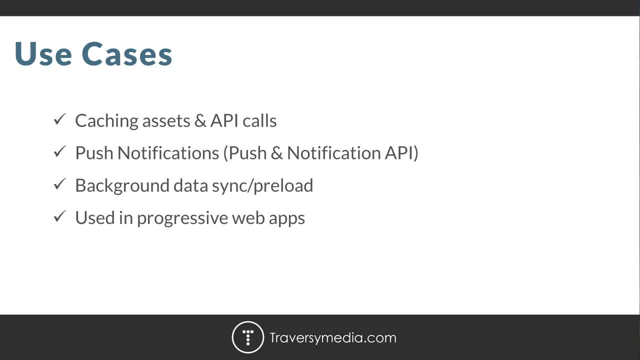 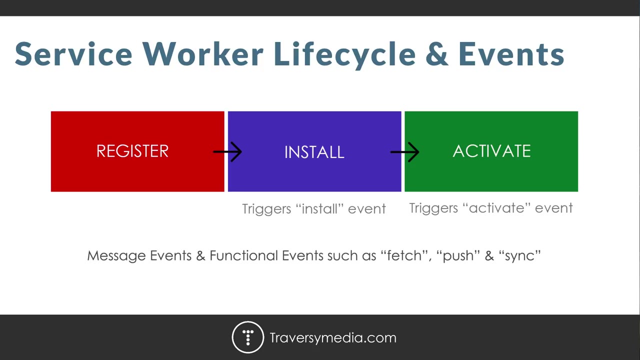 on hold in the cache until connectivity is restored, and then that post will get liked. Okay, So if you've ever used the Instagram mobile app, it works in a very similar way when it's offline. Now, Okay, So you should have something called a life cycle, and this is a very simplified diagram. 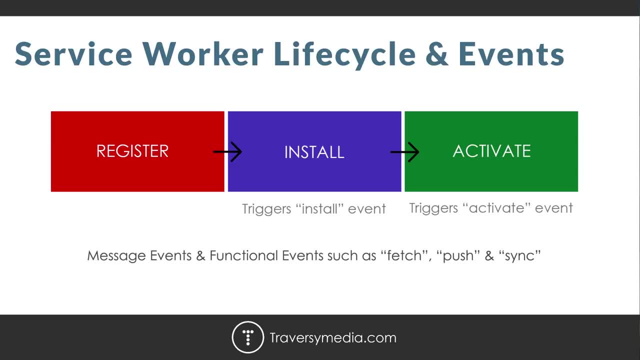 that I created. But basically the first step is to just register the worker. then you can install it by triggering the install event and then activate it using the activate event. After that it can receive message events and functional events such as fetch, which. 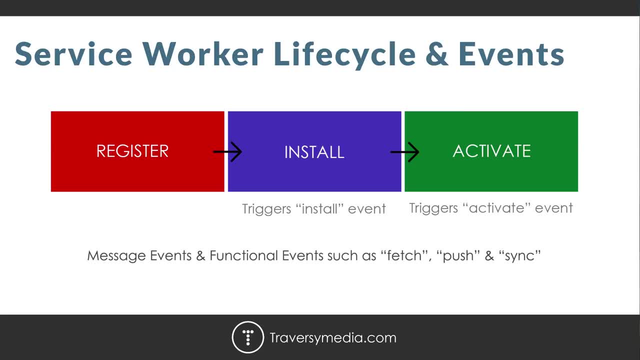 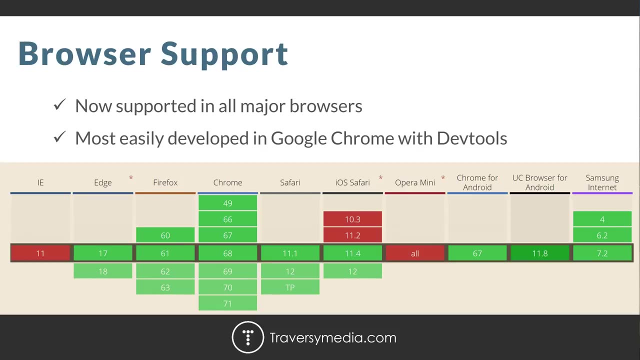 we'll be using, And then you also have push for the push notifications and then sync for the background sync API. All right, Okay, So enough will make more sense when we get into it, when we start to work with these events. Now, as far as browser support goes, service workers are supported in all major browsers. 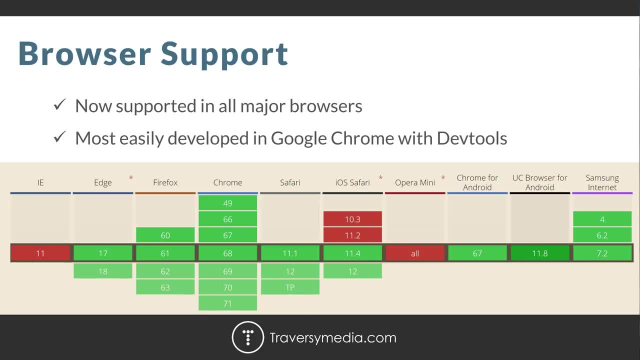 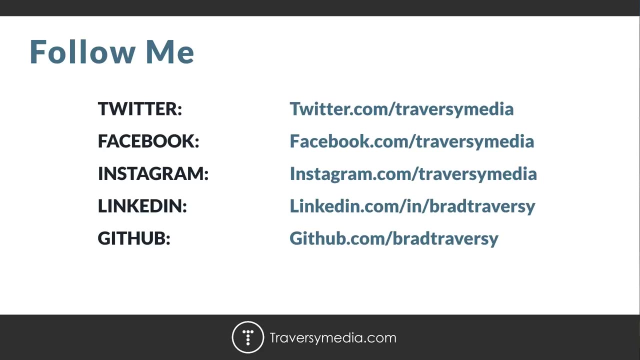 not Internet Explorer, but all normal browsers. However, the background sync API is not supported in Edge or Safari yet, as far as I know, But it shouldn't be long for them to adapt. All right, So enough with the slides, Let's go ahead and jump in and let's take a website. 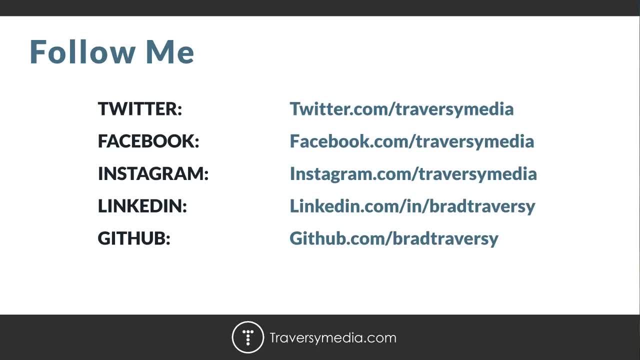 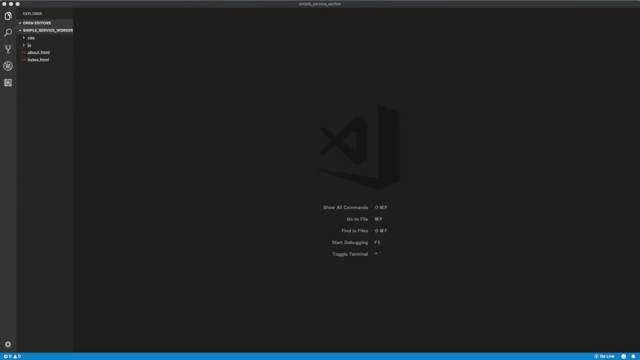 Let's add a service worker to it So we can cache it and we can have offline viewing of the pages. All right, guys, so we're going to get started now. I just have a very simple website that we're going to be working with. 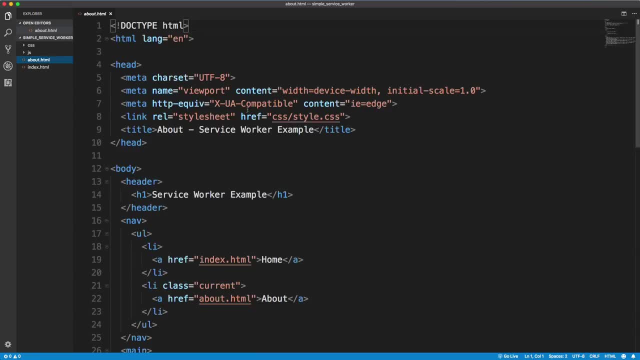 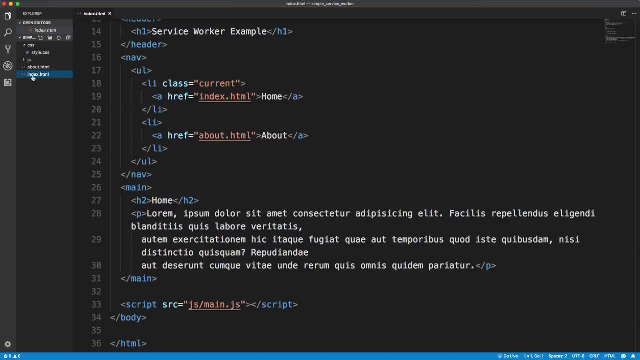 So we have just a simple index page and a simple about page and a CSS file with just a little bit of styling in it. So let's take a look at it. So I'm going to. I'm going to be using live server, which is an extension for VSCode. 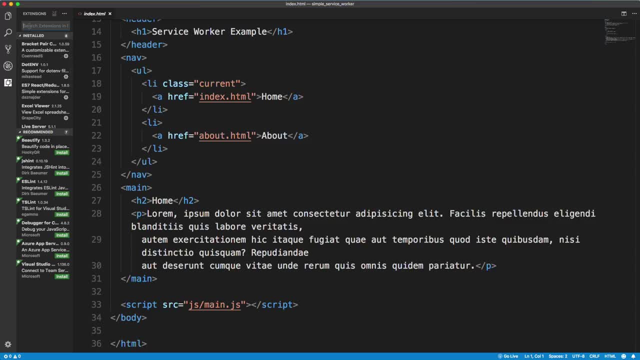 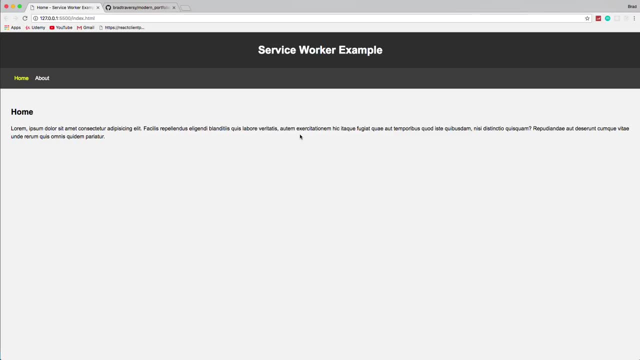 You can install by clicking on the extensions icon and searching for a live server and installing, And then you can simply say open with live server and it'll open on your local host on port 5500 by default. So this is our very simple website. 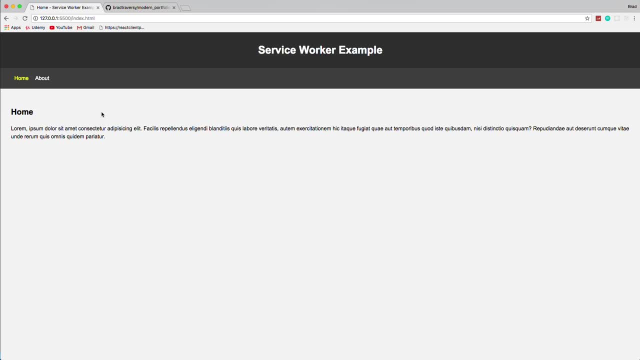 And the idea for this is that we want these pages to be available even if the user's connection drops. OK, and we're going to do that by create registering a service worker and also working with the cache. So I'm going to be opening my Chrome tools. 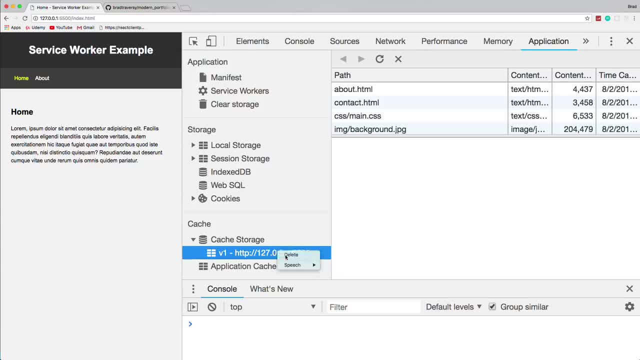 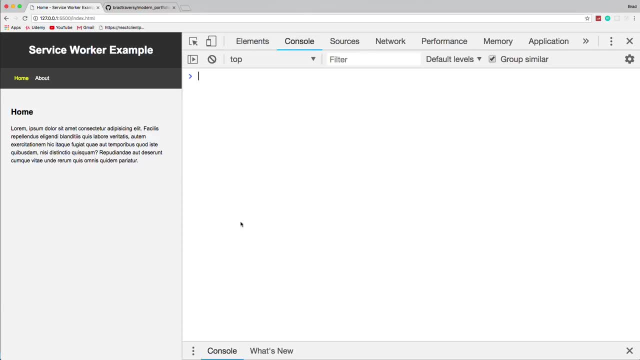 We're going to, we're going to work in here quite a bit. Let me just clear this cache out real quick, All right? So just make sure. OK. so right now we have nothing, No service worker registered. All we have is the files I showed you. 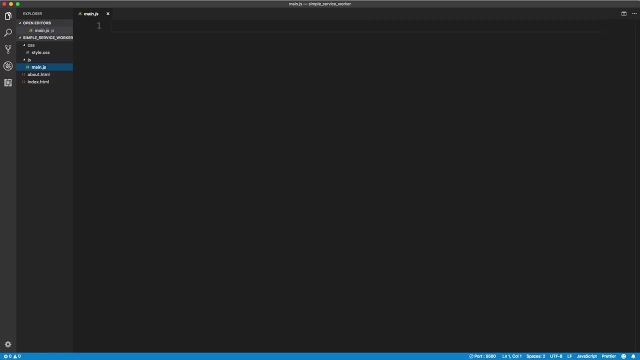 We do have a JS, a main JS file which has nothing in it. This is where we're going to register the service worker file. OK, so I'm going to create a file in the root directory. This is going to be our service worker. 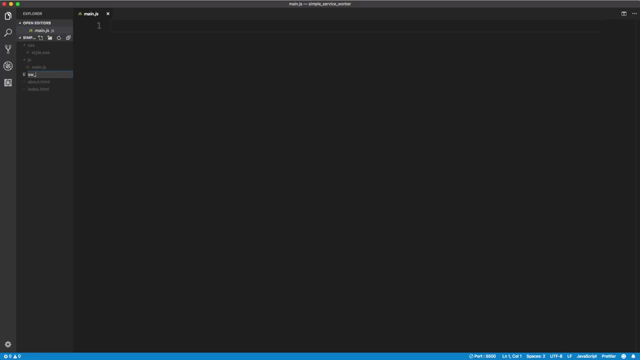 I'm going to call it SW underscore And let's call it cached. I'll say cached underscore pages dot JS. All right, so this is the actual service worker, but we have to register it elsewhere. Now you could do it in your HTML files, but you would have to put it in every single HTML. 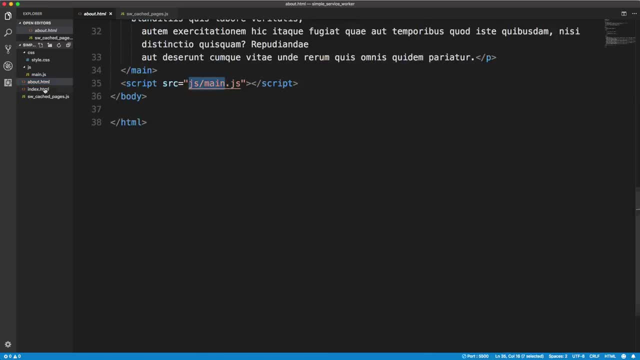 file, since the main JS is actually included in both HTML files. That's where I'm going to register it. OK, so we're going to go into main And In the very first thing you want to do is make sure service workers are supported. 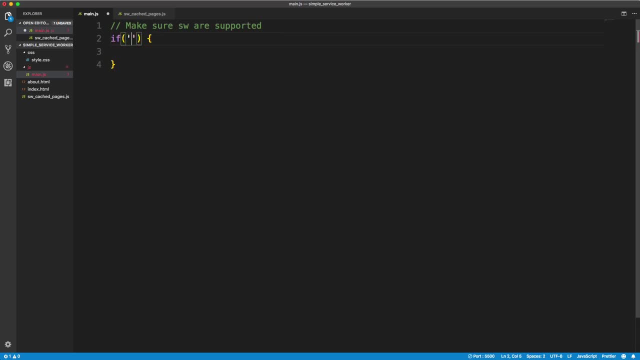 And we can do that with a simple if statement and we're just going to say if inside quotes service worker in and then navigator. navigator is basically like the browser object. You can also do if navigator dot service worker: OK, You can also do if navigator dot service worker in and then navigate to that object. 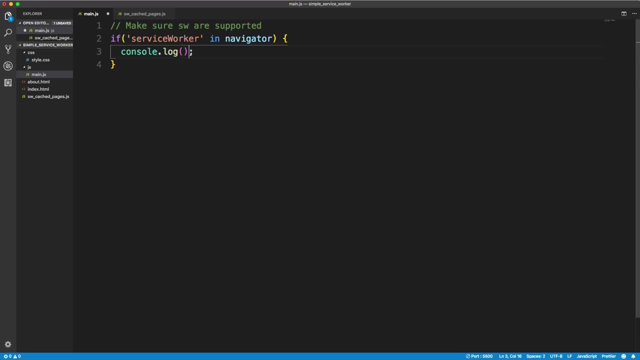 So let's just do a quick console log just to make sure I'm using Chrome. So obviously it is, it is enabled. but we'll just go ahead and do this anyway. So we'll say: service worker supported. OK, so we'll save that. 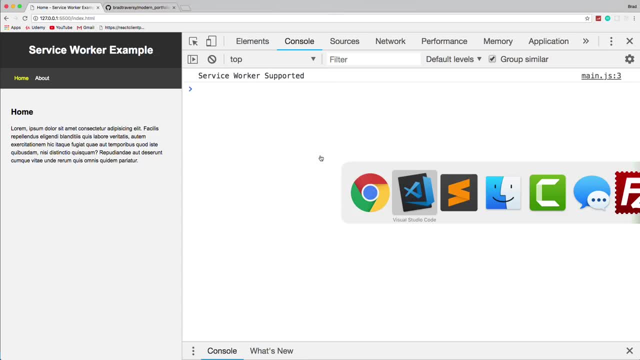 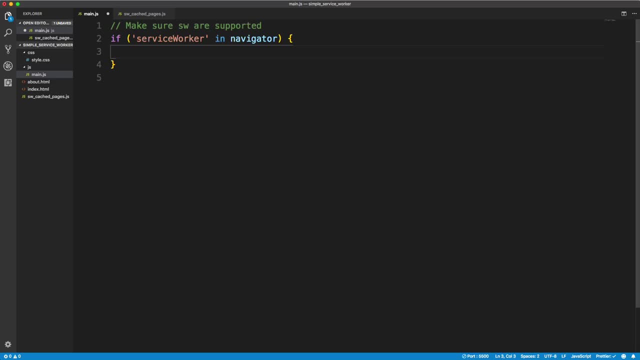 Let's go to our browser and we get service worker supported. Good, Now we'll go back. We can get rid of this log And we're going to register it now. We want to register it when the window loads, OK, so in JavaScript and in the browser we have a window object and we're going to call. 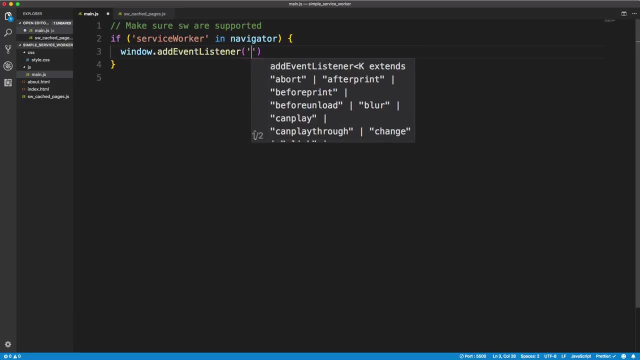 an event listener on it. with add event listener, We want to listen for the load event and then this is going to take a call back. You could put a function like this, but I'm going to be using ES6 arrow functions, So I'm just going to put a set of parentheses and then an arrow and then some curly braces. 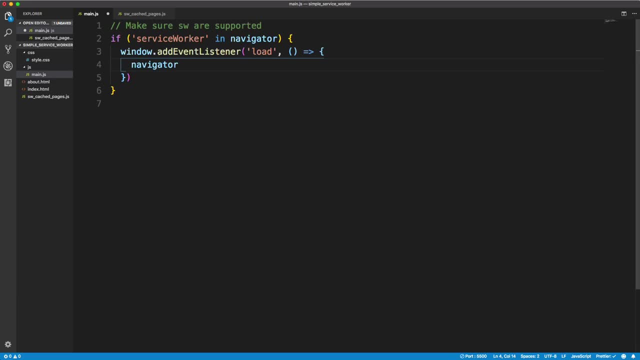 And then in here we want to take that navigator object and we want to say dot service worker. You can see I'm getting some dropdowns in VSCode here and we want to register it with dot register. So I'm going to go on a new line and say dot register. and then we want the file name. 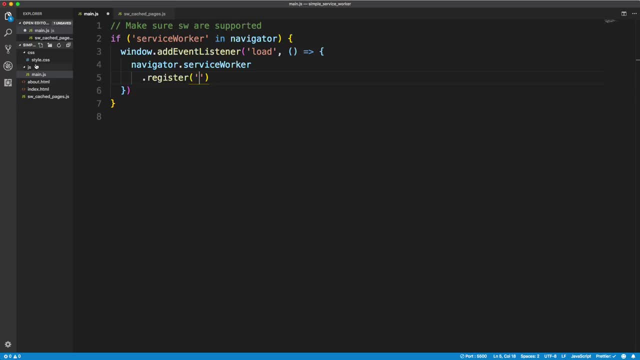 Now, since the file, the service worker file, is outside of the JavaScript folder, where we currently are, we have to do a dot dot slash and then the name, which is SW underscore. OK, Once we do that, that's going to give us a promise back. 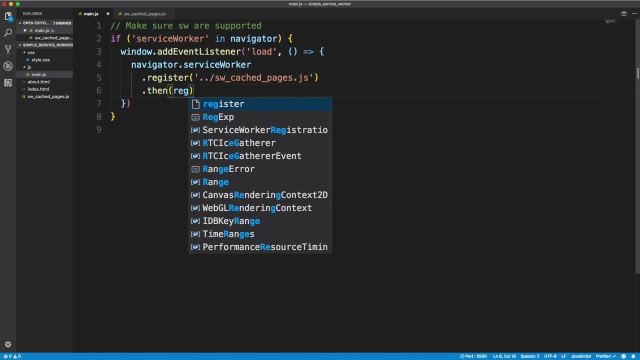 So we say dot, then it'll give us a registration object and I'm just going to go ahead and console dot log. here And again I'm using arrow functions, but you don't have to And let's just say here, service worker, and we'll say registered, like that. 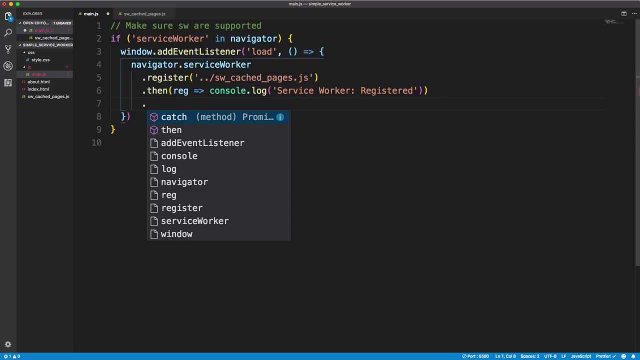 All right, And then if there's some, if something goes wrong, then that'll be in the dot catch. OK, that's how promises work. So in here let's just say it's going to give us an error and I'm just going to console. 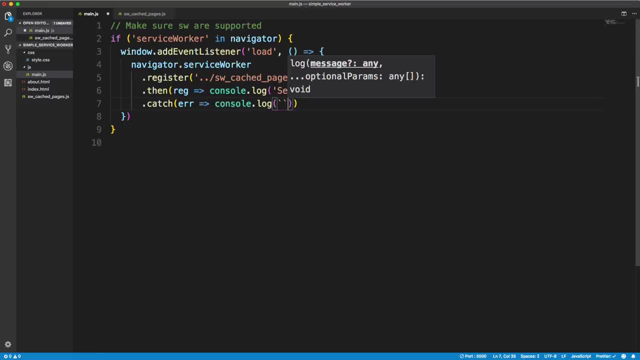 dot log. I'm going to put in back ticks here instead of single quotes, because I want to include that error variable. So I'm going to say service worker and let's say error colon, and then to put a variable in with. So that's going to give us a template string. 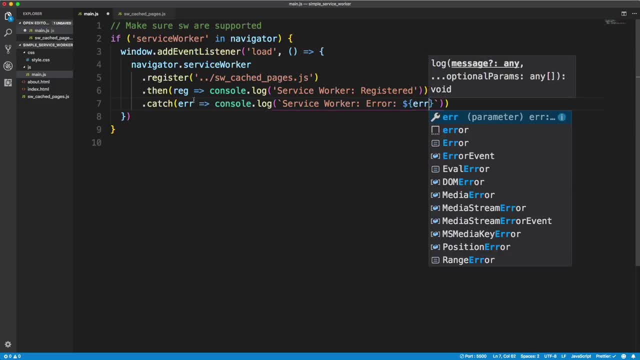 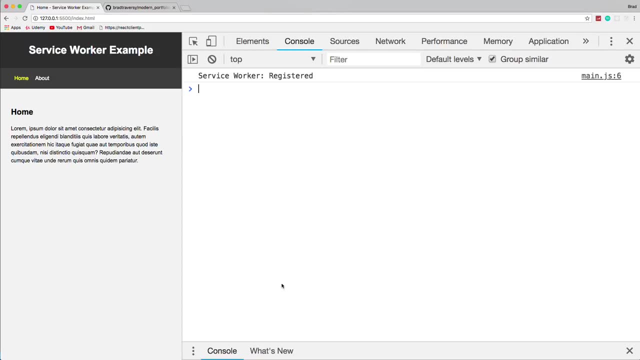 We can just go like that and we can simply put in the error variable that it gives us back right here And that's it. That'll register the worker. So if I save this and we go to Chrome, you'll see service worker registered. 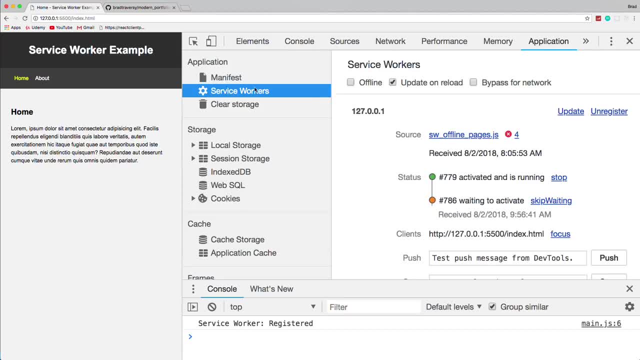 OK, And if we go to our application tab and go to service workers, you're going to see it here And it says SW offline pages dot JS. That's the name of the file- activated and running. It's actually waiting to activate. 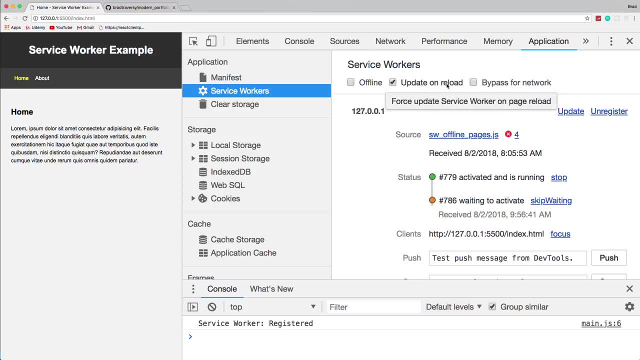 So just ignore that. If you see that, for now we're going to take care of it. And then this update on reload. make sure that this is checked, because you want to force the update on page reload. So let's go back to VS. 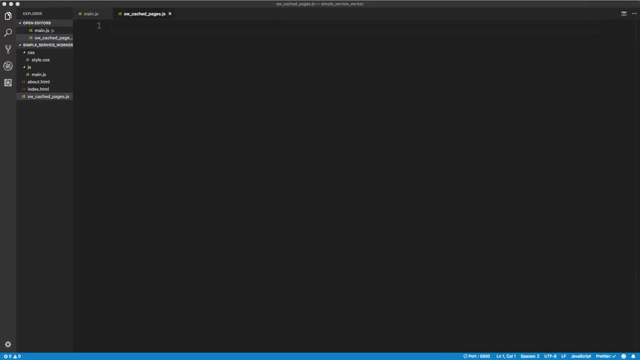 Code now and let's head into our service worker And in here let's see we're going to, let's call the install event. So say, call, install event. And to do that we need to attach an event. listener to the actual worker and we can. 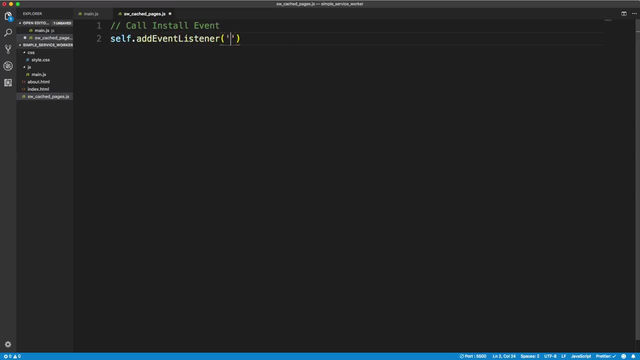 do that by saying self dot, add event, listener And we want the install event And that'll we get a callback here. You can use function if you want, But again I'm using arrow functions and this takes in an event parameter. So you want to pass in E or you can do event or whatever you want to do. 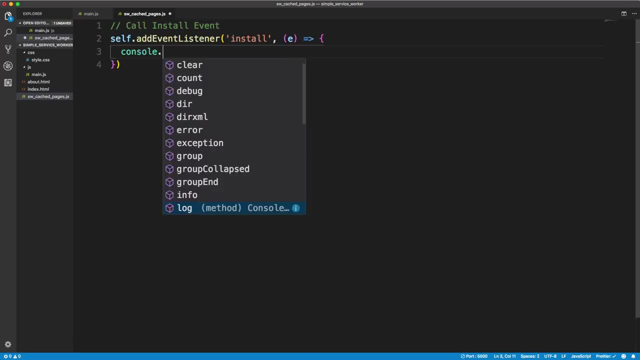 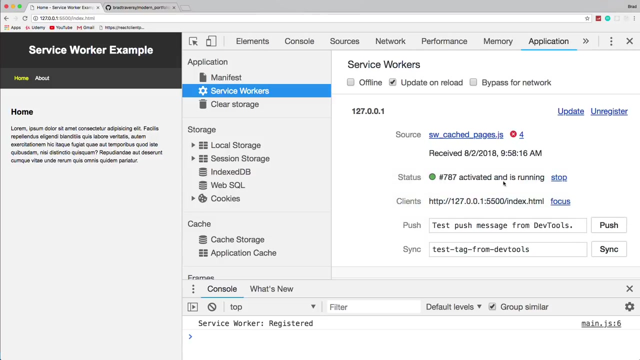 But I like to use just to eat. And then let's do a console dot log here And let's say service worker and we'll say installed. and this should have quotes around it, Sorry. OK, so we'll save that. and let's go back to Chrome and now you can see it says activated. 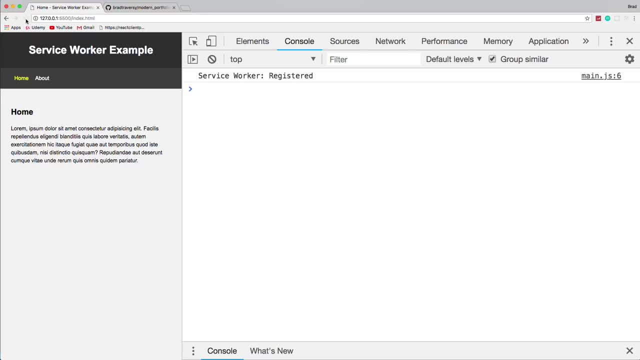 and running And if we go to our console, if I reload Italy, you might see it flash, The installed message. See that flash. If you want to actually see it, you can go to the little gear and preserve your console log and then reload. 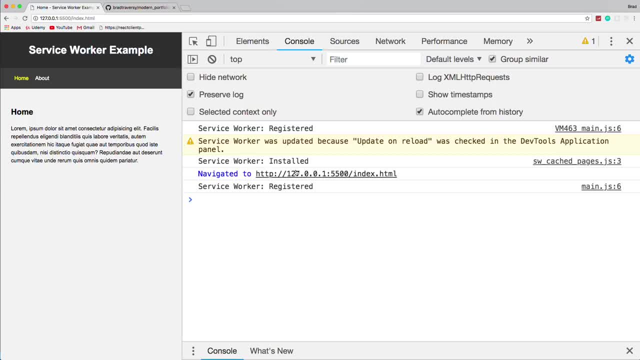 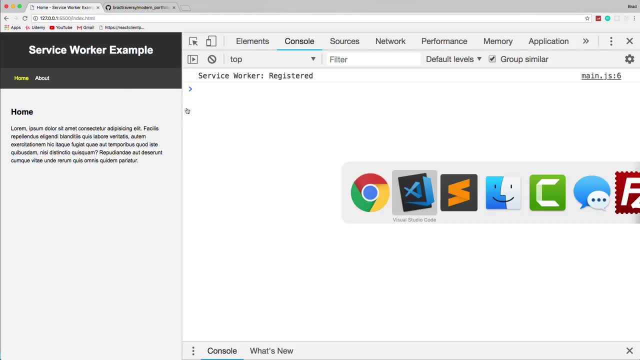 And now you'll see the service worker installed. OK, so it just gets installed really quickly and it just flashes. But you can see it if you preserve your log. So that part's done, at least the in the install. We have to do some stuff in here, but at least we have the event. 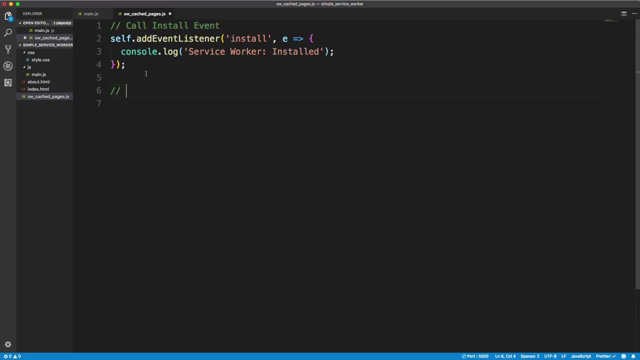 Let's now call the activate event. Actually, I'll just copy this here And let's say: call activate event, So this will be activate. And then we'll say service worker activated. OK, remember that life cycle I showed you in the slides. 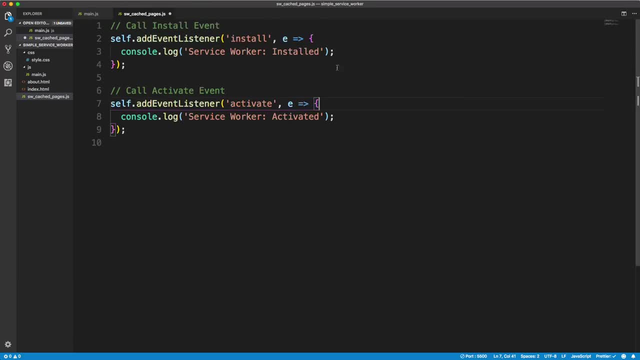 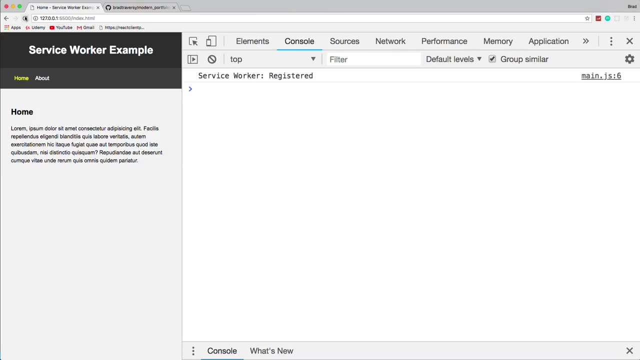 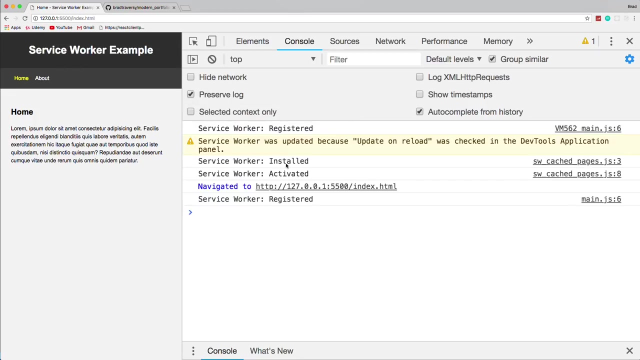 We have the register, which happens here, and then we have the install and then the activate. OK, so if we take a look at that- and there's certain things You do in certain areas and so I should say in certain events, So if we preserve the log and reload, you'll see installed and activated. 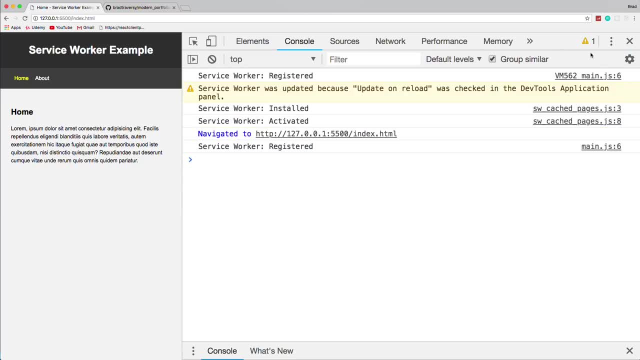 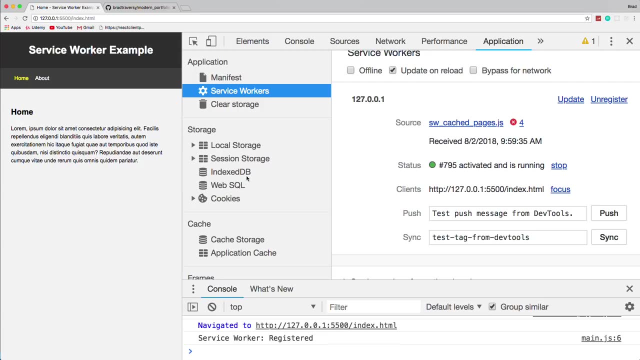 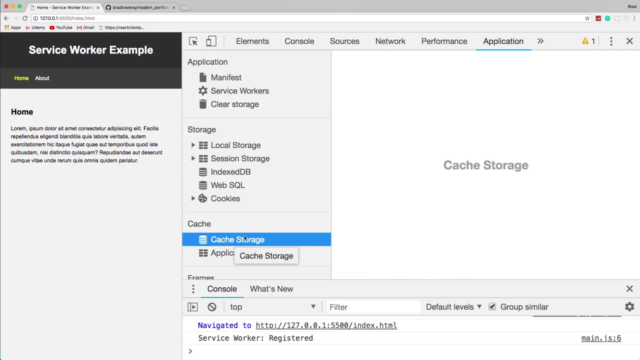 OK, let's go ahead and uncheck that, and everything should still be OK here. Good, Now this is another tab. we're going to be paying attention to cash storage. when we actually do cash something, It's going to be put into here. 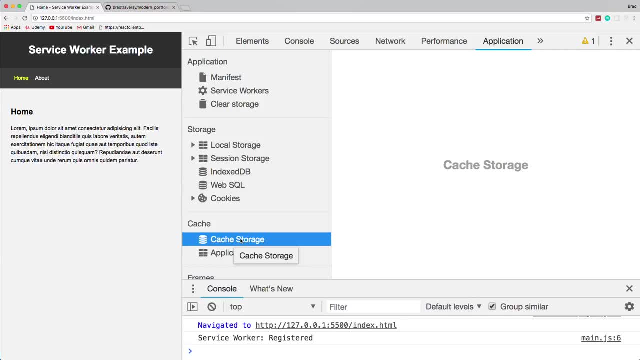 And then We have access to this even if the connection drops and there's no internet connectivity. and that's that's the beauty of of working with service workers and cash. And that's why it's important for progressive web apps, because you want them to work more. 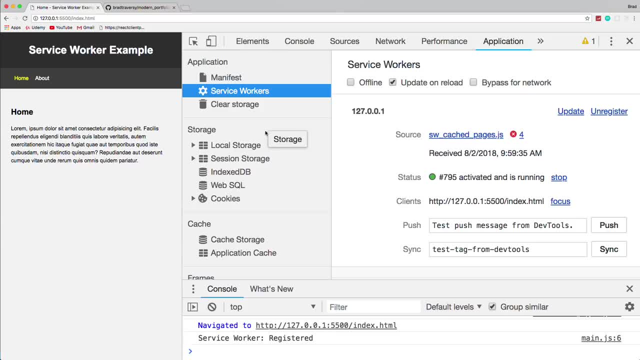 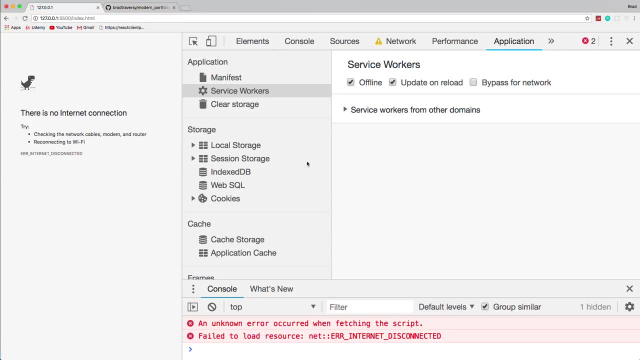 like native apps, and in most native apps, even if the connection drops, it doesn't just go blank. It doesn't do this. If I check offline, they reload. We get this. OK, And this- this is this- will simulate offline. 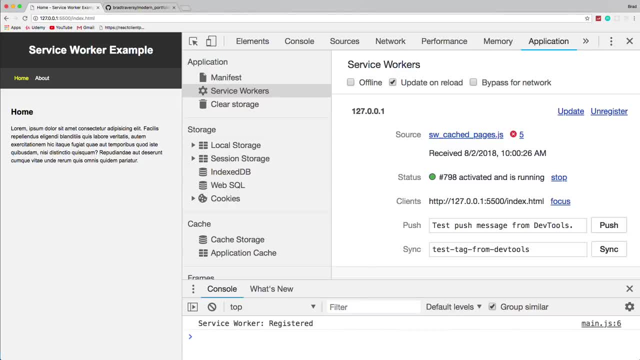 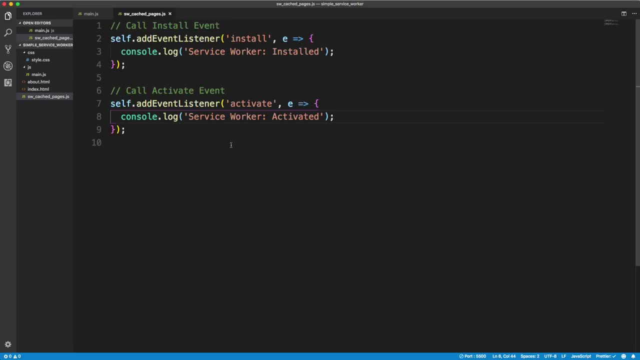 OK, You know for the if the connection had dropped, All right, So let's go back to our service worker file. And now we're going to think about caching. So we're going to cash all of our pages. We're going to need the assets and the actual HTML pages. 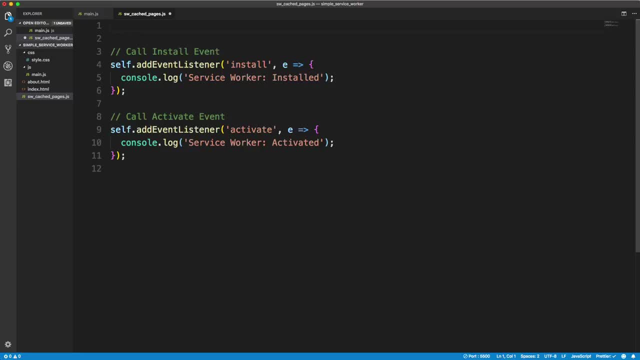 And I'm going to give you kind of two ways to do it. First I'm going to show you how to cash the individual pages, and then I'm going to show you how to actually cash the entire response that we get. OK, So the entire website or page. 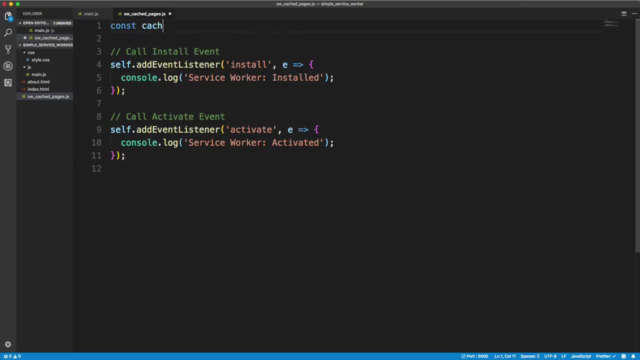 So let's create a video, Let's create a variable up here. We're going to call it cash name. That variable can actually be whatever you want. This can also be whatever you want, But a lot of times you'll see like V1 for version one, because you might have different. 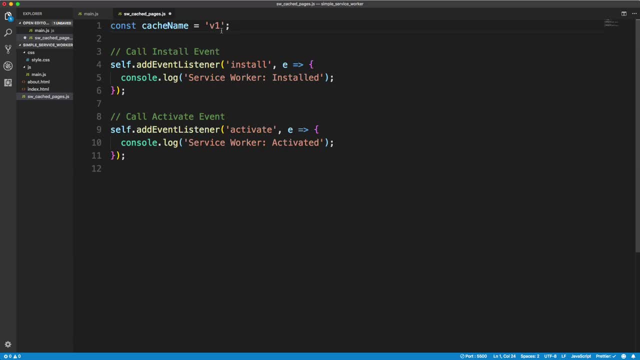 different sets of caches and you want to keep track of them, So we'll call this V1.. Then we need to create a variable of assets, So we'll say cash assets, And this is going to be an array of all of our pages. 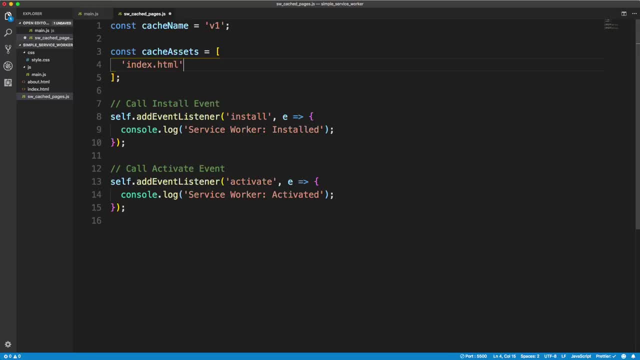 So we have index dot HTML. We have about dot HTML. OK, We have a CSS file which is in the CSS folder, So CSS, slash, style dot CSS. And then we have our JavaScript file, So let's say slash JS, slash main dot JS. 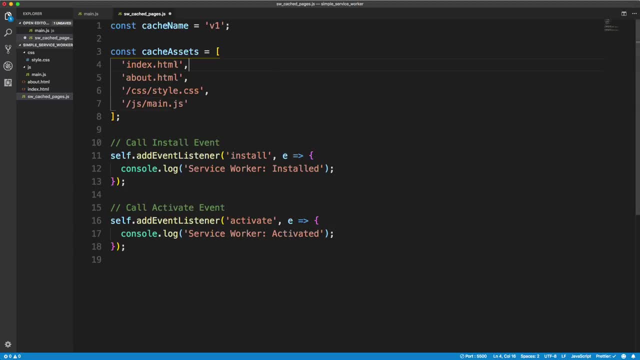 So those are the assets that we want to cash, And there's, There's not. There's not a lot in this little website. So this is a fine method to do this, But if we had a ton of pages, then we might want to do the second thing I'm going to show. 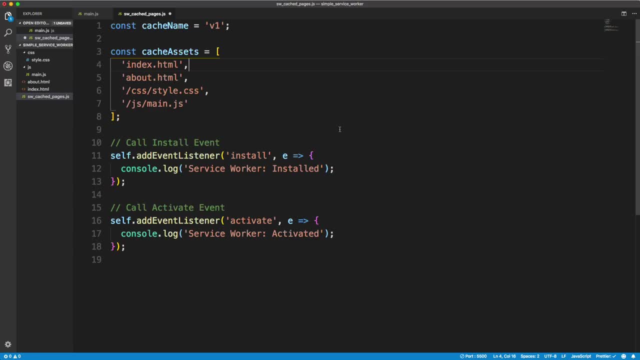 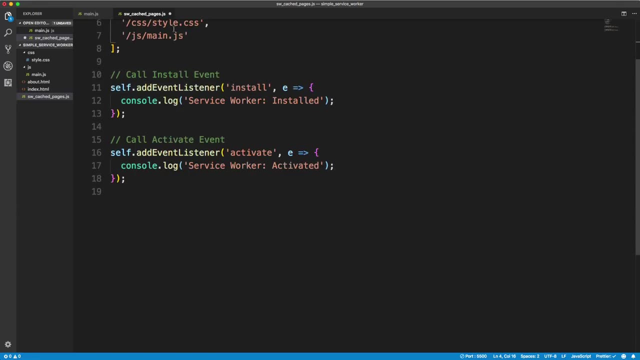 you, which is basically just taking the entire response and caching it. But for now we're just going to do this And then in the install event is where we want to handle caching these assets. So I'm going to go into this console log, I'm going to leave the console logs, just to kind. 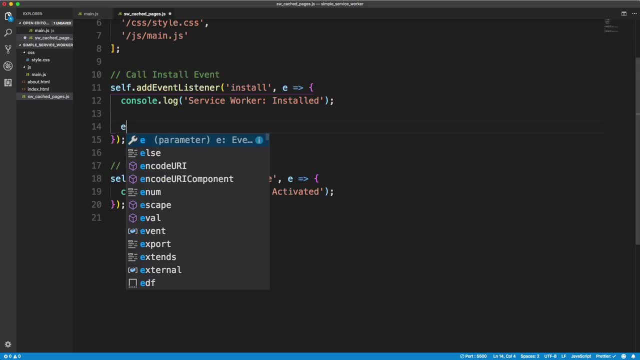 of map, what's going on. But under here we want to say: you want to take that event And we want to call wait until OK, which basically is just telling the browser to wait until our promise is is finished, until it it it gets rid of the service worker. 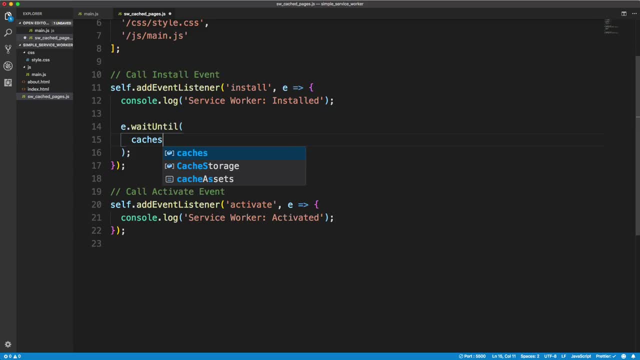 So in here we're going to be using the caches storage API. So we're going to say caches dot open, which opens a cache, and I'm just going to put this on a new line. So it opens a cache and we want to pass in our cache name that we defined above. 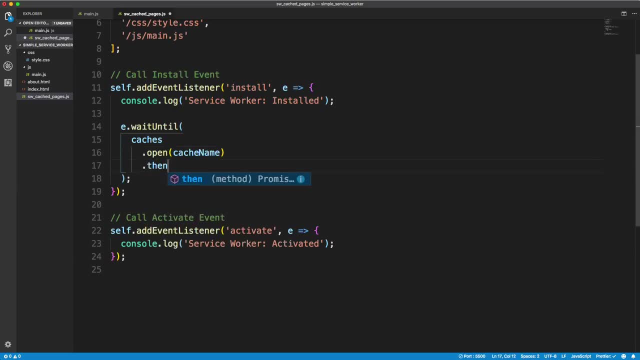 OK, Now, once we open it, it's going to give us a promise. So we want to do dot, then it'll give us a cache object and then we want to take that. and I'm actually going to put some curly braces here because I want to do a console log, just 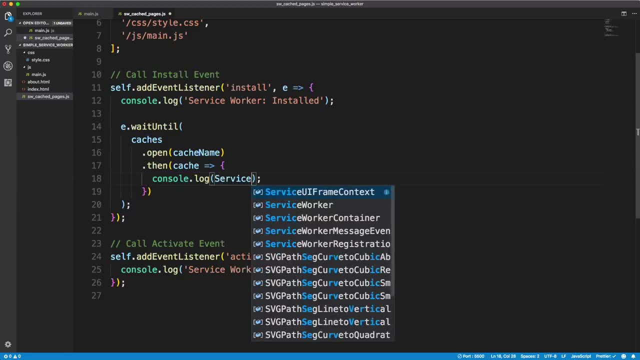 to to kind of map what's going on. We're going to say from the service worker: So whoops. So why do I keep forgetting these quotes? So from the service worker, Let's say caching files, because that's what we're going to do and we're going to take. 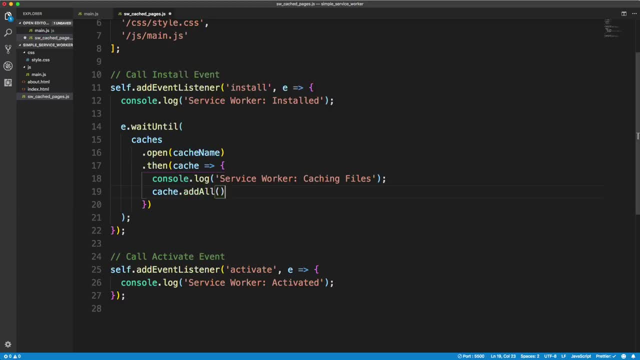 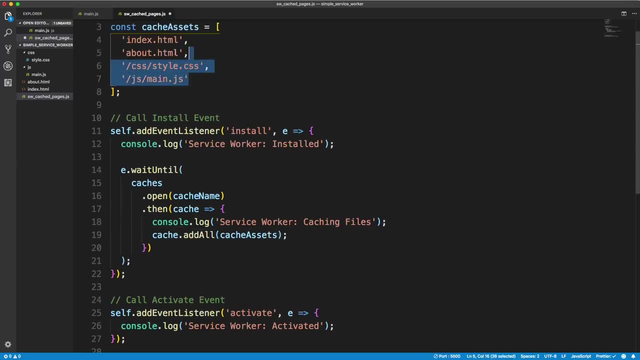 that cache object and we're going to call method, called add all, and inside here we want to place in our assets that we want to cache, which is cache assets. That's the array. Sometimes you'll see people just put the array directly in here, but I like to define a variable. 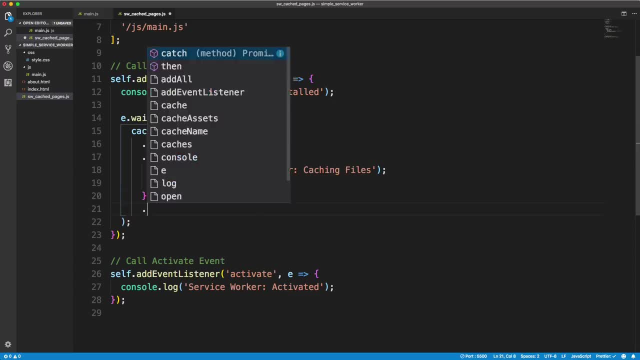 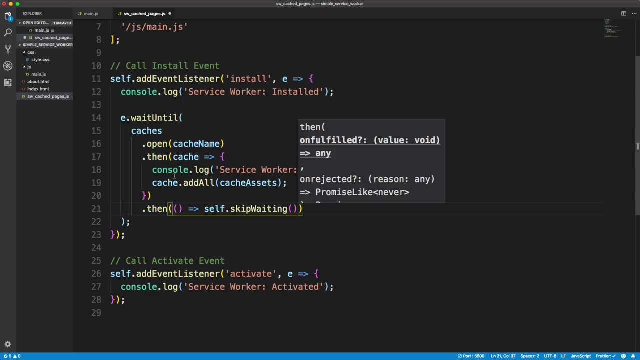 up here and then put it in, and then we just want to add another dot then. So when everything is all set, we can skip waiting. So we can just do a function in here. I'm going to use an arrow and we can say: self dot, skip waiting, like that. 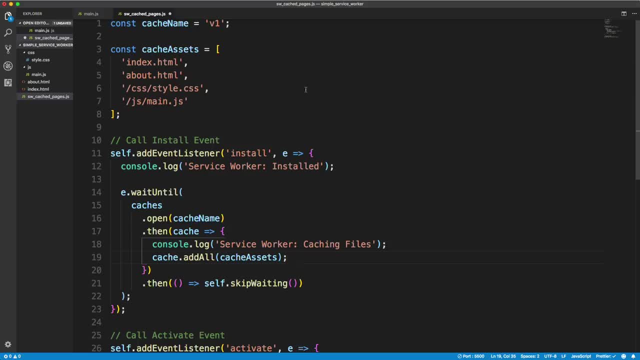 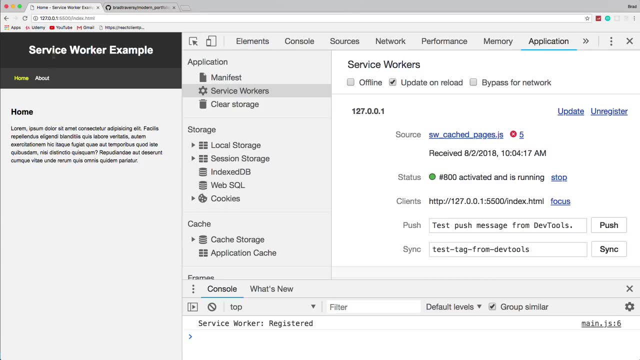 OK, so that should actually put the files in the cache. So I'm going to save this and let's head over to Chrome and it already reloaded. but I'll just go ahead and reload again. And now notice that down here under cache storage is an arrow, and if I click that, we'll. 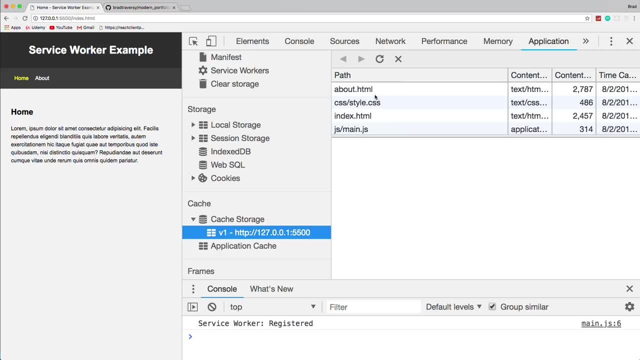 see our version one, And Now on that it's going to show us all the files that have been cached, which is basically our entire Web site. the HTML, the CSS and the JavaScript gives us the content type, the size and the time or the time it was cached and it's now there for offline viewing. 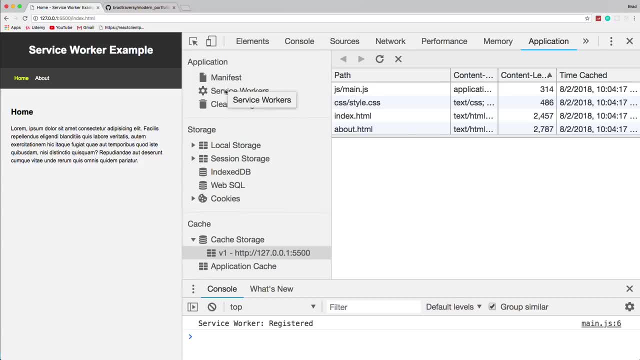 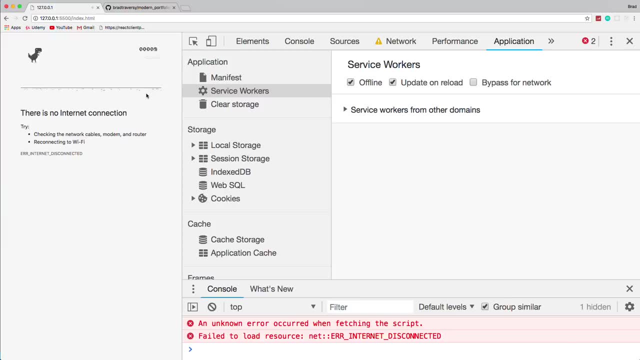 Now, we haven't set up that part yet. If I were to click offline here and reload, we're still going to get this, this here. I mean we can play this, this cool little game here. I know this is, this is hours of fun, but you know it does get old after a while, so we're probably going to want to show the. 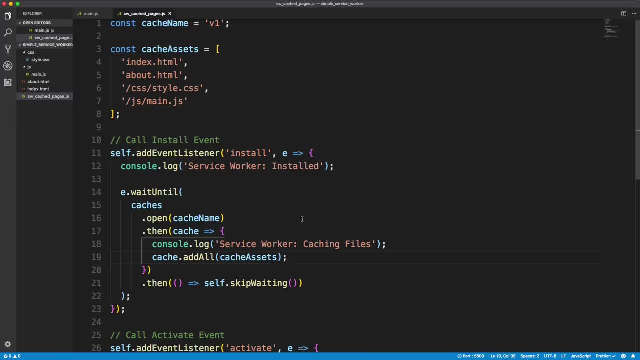 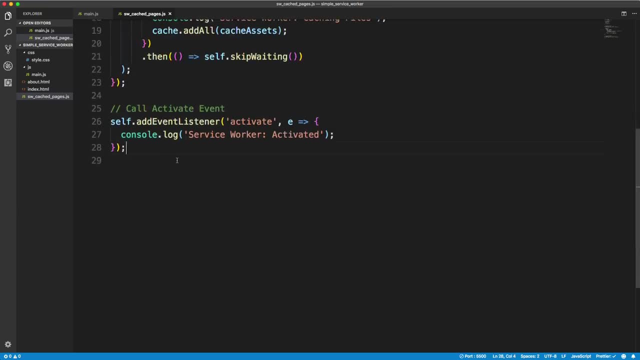 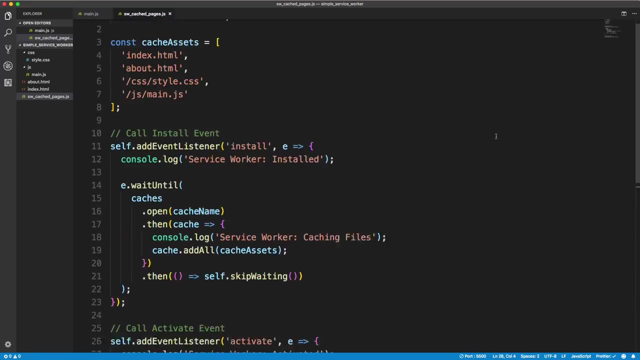 Web site. So let's go back and where we want to do this is in the fetch event. OK, but actually before we do the fetch event, let's use our activate in the activate is where we want to clean up any old cache. So if I change this to like V2, actually I'll show you real quick if I change it to V2 and 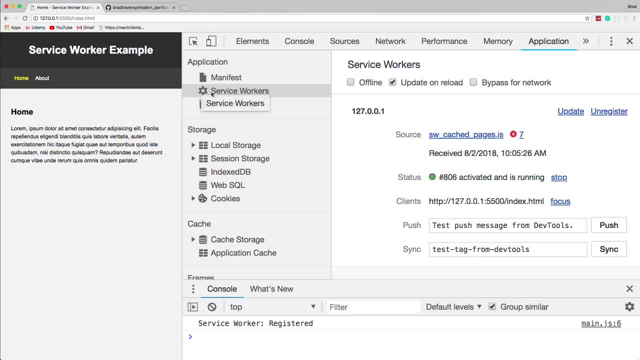 I save it. Let's go and we run this, we reload and let's look in cache storage and we have V1 and V2 in here, All right. So what we want to do is we want to get rid of any unwanted caches. 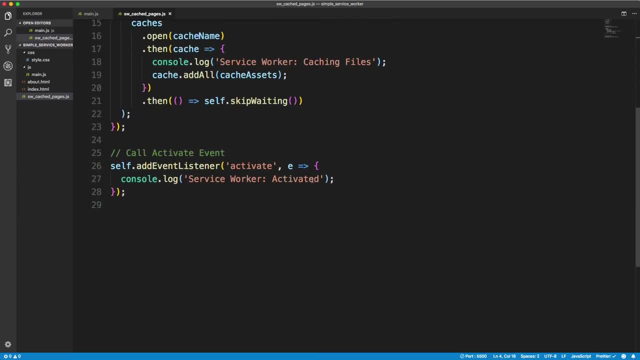 So that's, that's where we do. we do this in the activate event. So under this console log let's say: remove unwanted caches. So again we're going to do our E Dot, wait until. and in here we're going to say caches, dot keys. 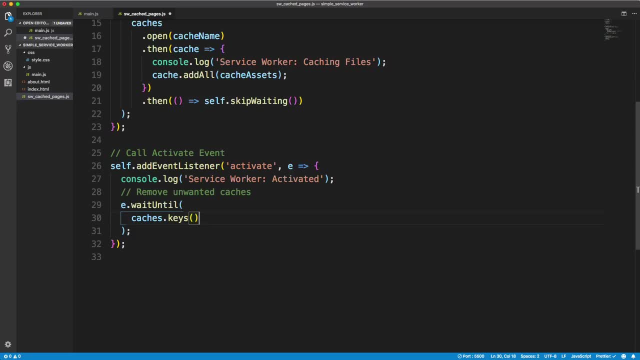 So what? the what we're doing here is we're going to loop through the caches and we're going to have a condition that basically says, if the current cache isn't the cache that we're looping through the current iteration, then we want to delete it. 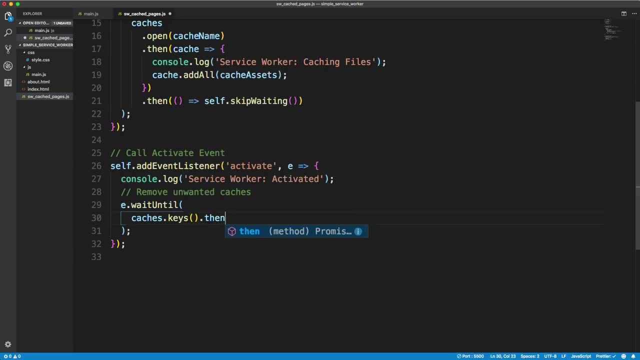 OK, So to do that, we do a dot, then here- because this gives us a promise- the cache dot keys And Inside here we're going to say cache names. OK, So for each one we'll call this cache names and we're going to actually have to return. 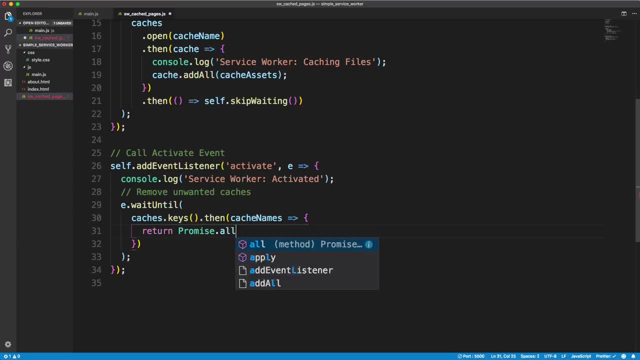 a, we're going to do promise, dot all, And inside here we're going to take the cache names. so, cache names, and we're going to map through them. OK, Map is just a high order function included in vanilla JavaScript, And then for each one we'll call it cache. 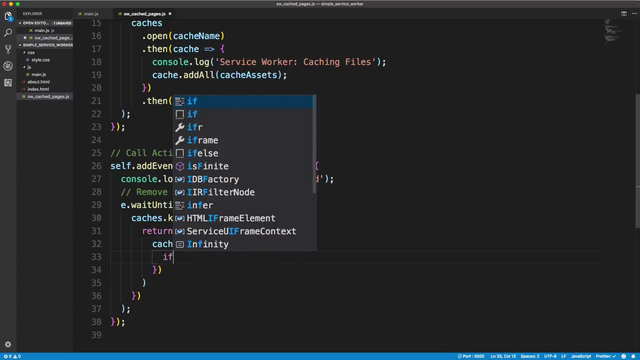 And let's put an arrow function here and let's do a conditional so we'll say if. Let's say if the cache is not equal to the cache name, OK, So basically, if the current cache we're looping through is not equal to whatever we have here. 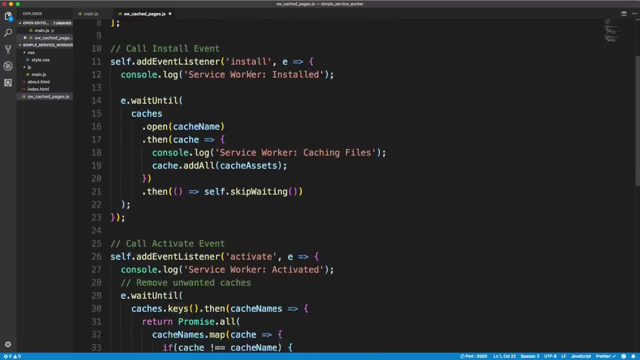 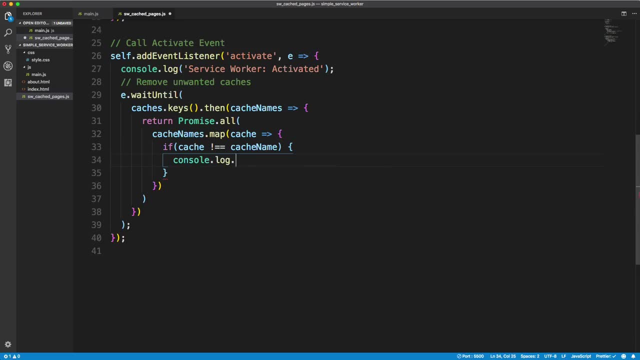 in this case V2.. I'm actually going to change it to V1.. Then what do we want to do? We want to delete it. So I'm going to put a console dot log here And I'm going to say: see, service worker. 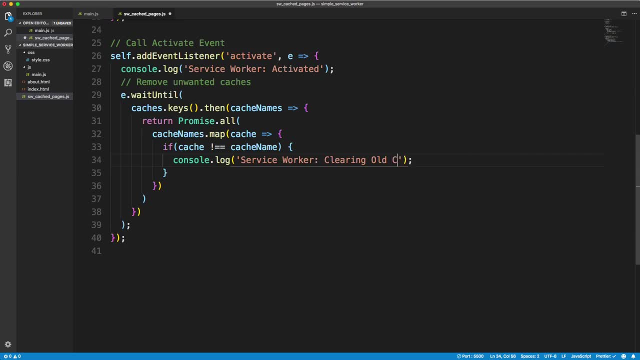 Say service worker, and we'll say clearing old cache, OK, And to do that we simply need to return caches, dot delete OK, And we want to pass in whatever the current cache is, as long as it's not equal to the cache name, which is the current cache we're dealing with. 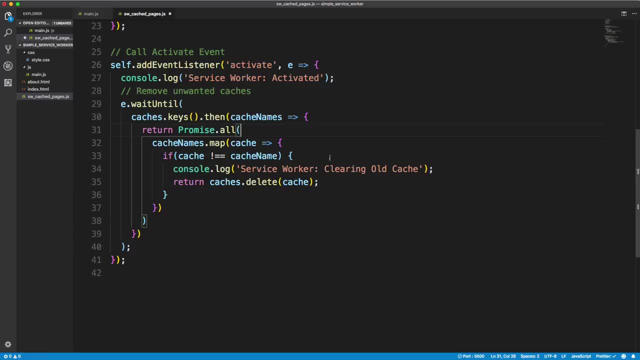 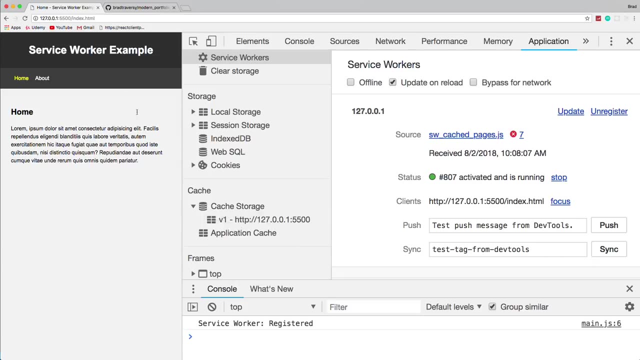 OK, And you could use filter here as well, but it's fine, I'm just going to do it this way. So let's go ahead and save that and it reloads automatically with live server. so I shouldn't have to reload and you can see that now. V2 is gone. 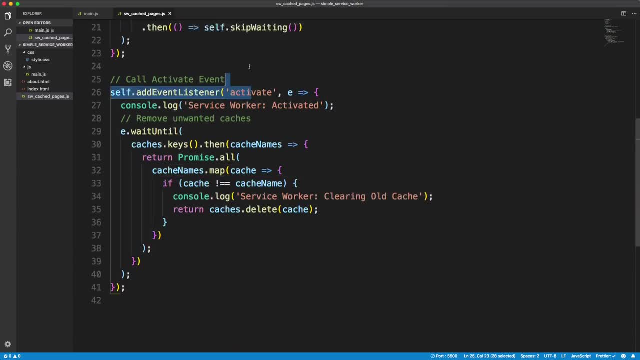 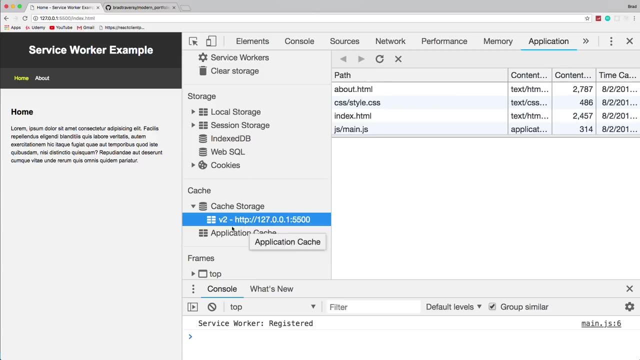 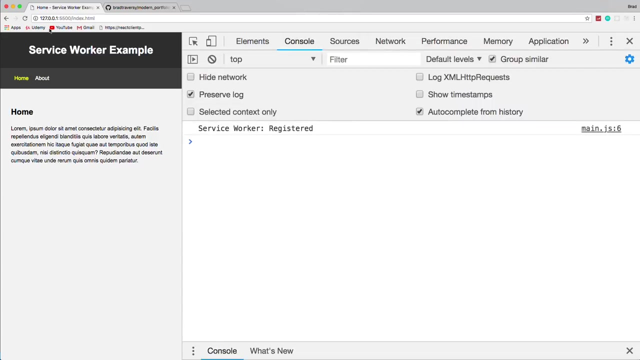 Now, if I see the V1 here, if I go and change this to V2. And save, and we go back. Now V2 is there and V1 is gone And if we want to look at the console log, will preserve the log and reload. we'll see. 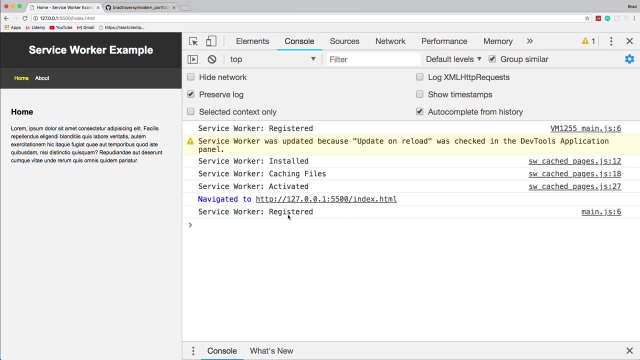 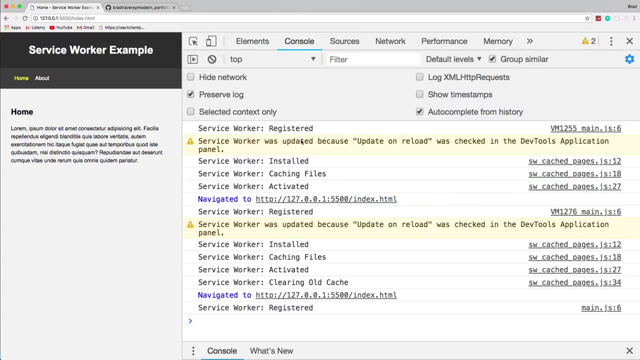 installed caching files. Actually, we don't see the message that it's getting rid of the old cache because I didn't switch it. But if I go ahead and switch it back to V1 and save now, you'll see right here clearing old cache. 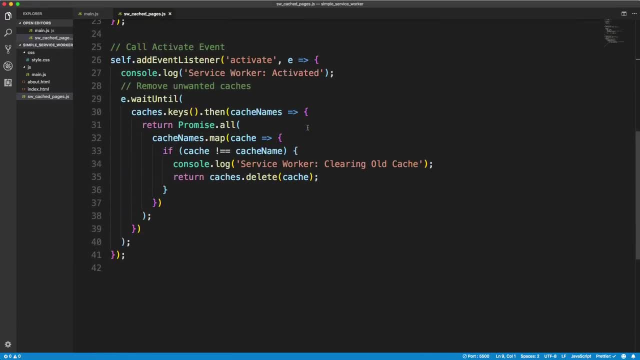 OK, OK, So that's. that takes care of that. Now we need to be able to show our cache files if we're offline. So that happens in the fetch event. So let's say call fetch event and we're going to say self dot, add event listener and we 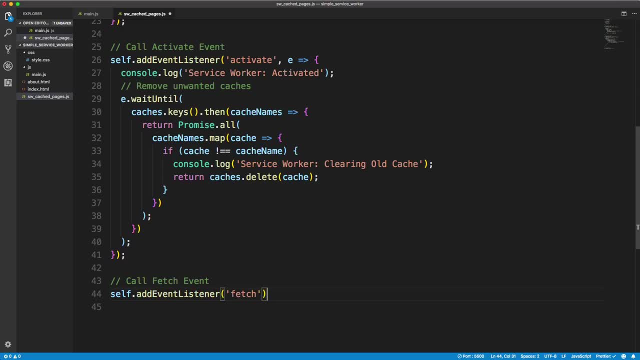 want to listen for fetch. So whenever the request is made, this should fire off and we can intercept it however we want. So let's remember, I showed you the image of the service worker in between Chrome and the server. That's, that's what, what we can do here. 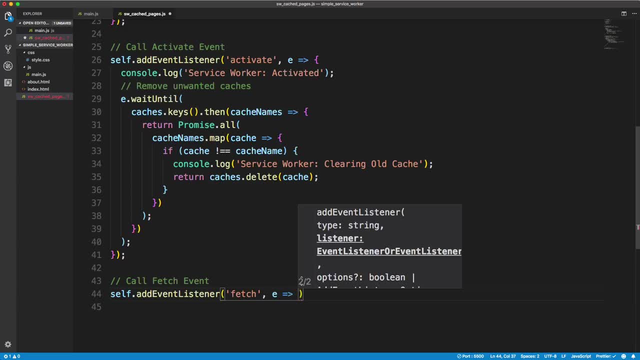 So we're going to pass in a callback with an event parameter and let's just do a console dot log. I know there's a lot of console logs, but I want you guys to see the process of how everything works. So let's say service worker and we'll say fetching. 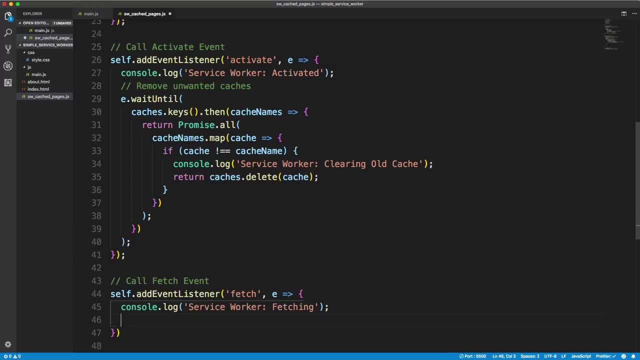 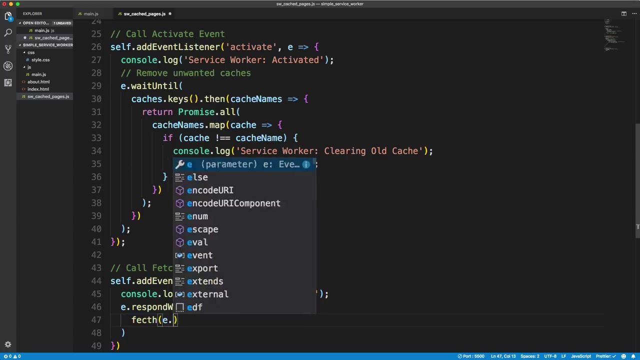 And then we want to First check if the live site is available. if not, then we want to load the cache site. So we say he dot respond with, And in here we're going to do fetch to put this on a new line. So in here let's say fetch, and what we want to fetch is the initial request. 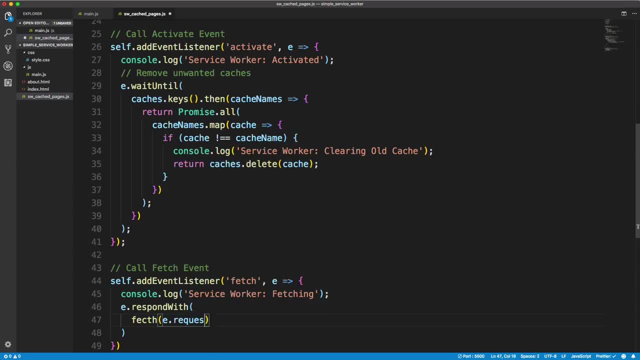 So you can get that with the event parameter dot request. All right, Now if this, if there's no connection, then this is going to fail. And since this returns a promise, if it fails and it's going to be in the dot catch, OK. now if there is a, if there's a dot catch, then we want to put a function in here. I'm 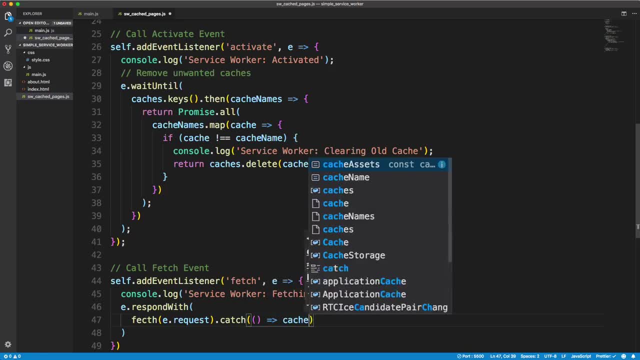 going to use an arrow and I'm going to say caches, dot match, OK. so basically, what I want to load from the cache and I want to put in a dot request and this will be from the cache. So the files, whatever we're looking for, such as index HTML about HTML, it'll load it from. 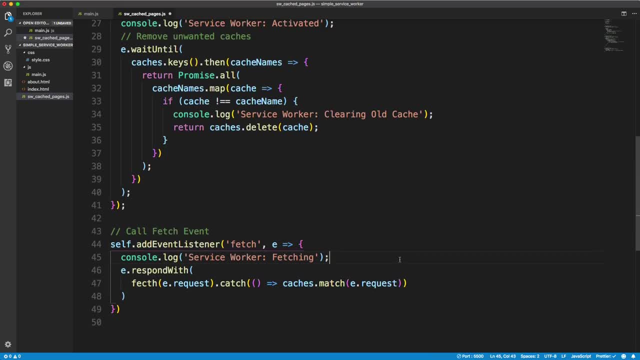 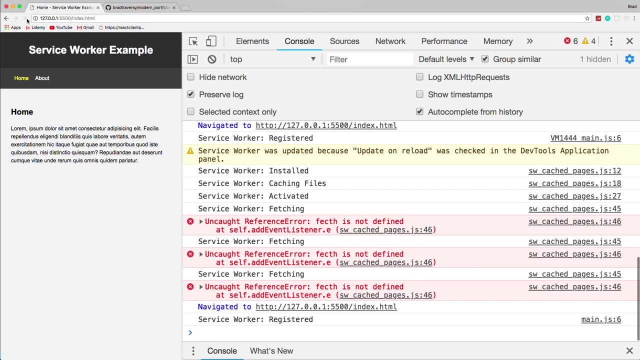 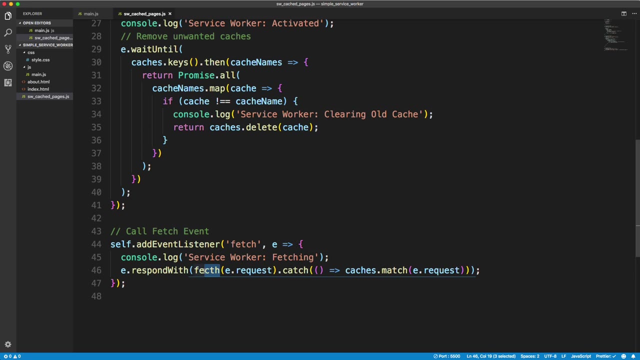 the cache with this, this dot match method. OK, so hopefully this works. Let's go ahead and save it and let's go back to Chrome and we'll reload. Whoops, I spelled fetch wrong, Course I did. Things are going too good. 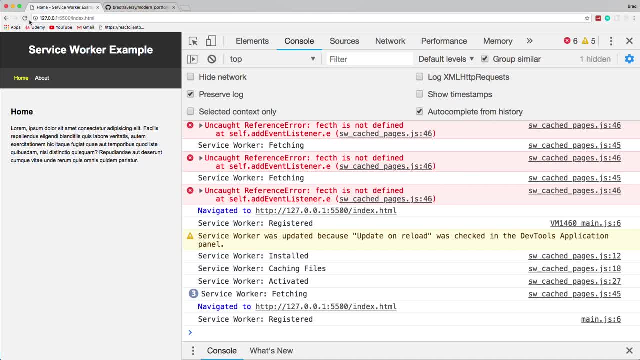 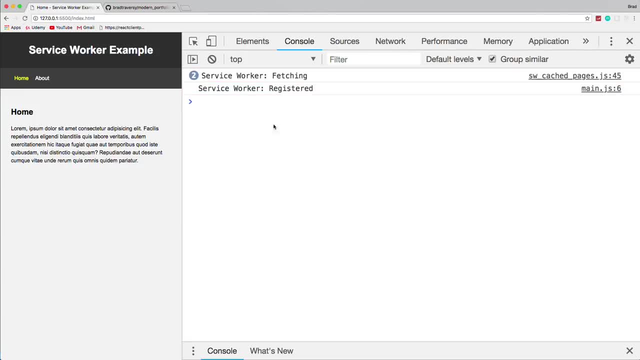 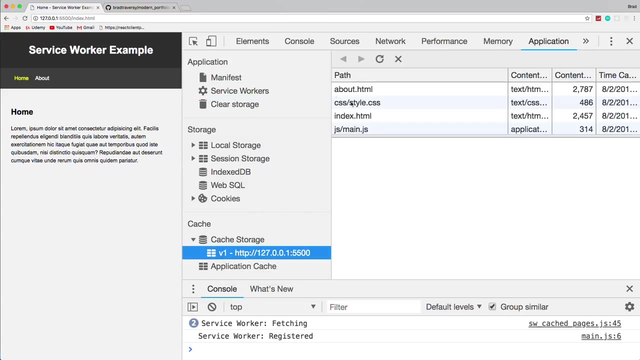 So fetch and Let's reload here, OK, and let's preserve the log so we don't have all this crap here. And then we'll go to our application and let's look at service workers and let's look in the cache. We still have all of our files here. 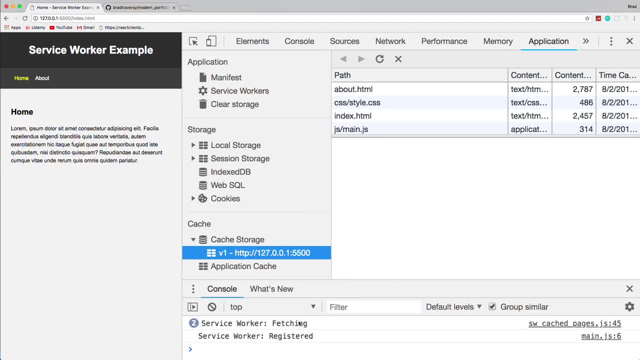 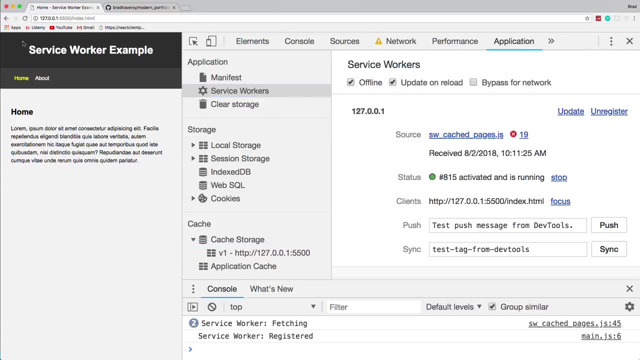 Now, since we have that fetch event- you can see it says fetching right here- We should be able to see the site even if we're offline. So let's go to service workers and check offline and reload, And there it is OK. so we're- we're technically offline right now. 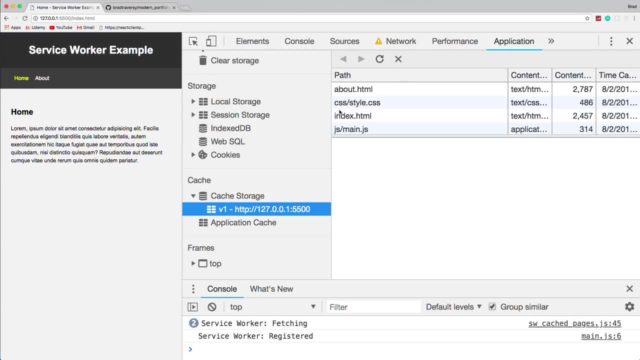 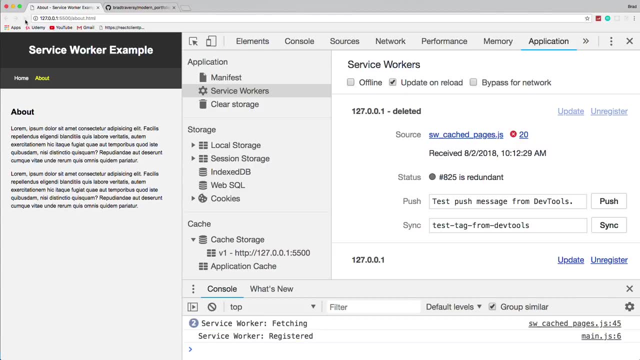 Now, if this, this is what's being served, it's not coming from the server, so it doesn't matter if our connection drops, All right, so let's go ahead and put this back online and reload, and now we're back online, All right. so that's, that's one way to do it. 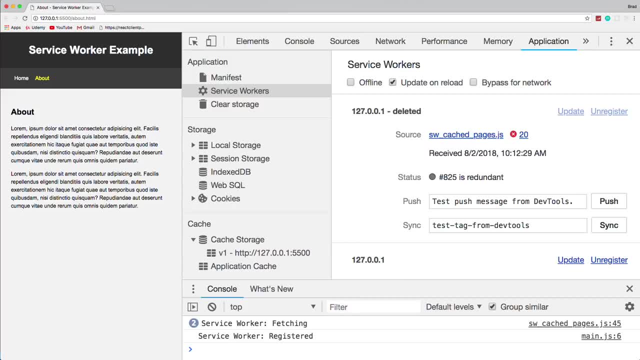 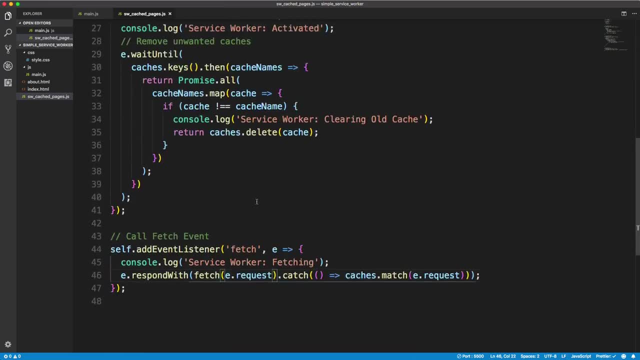 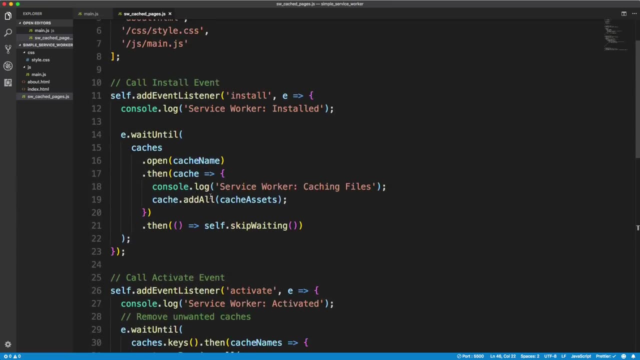 I don't know why this tab is open now. Like I said, if you want to cash the entire response, you can do that, But you do that in the actual fetch because you need to first fetch the response and then cash it, as opposed to, you know, doing it up here in the install. 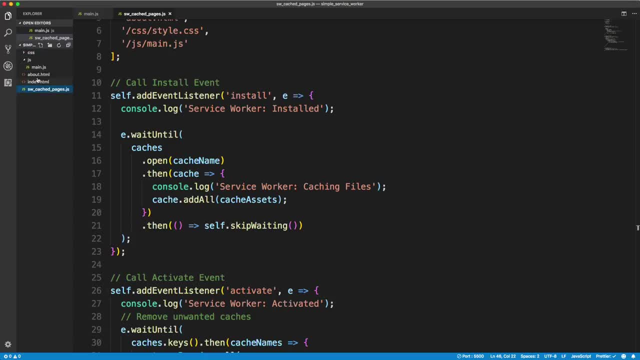 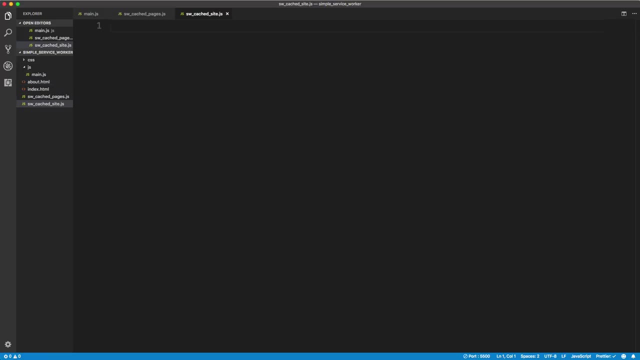 So I'm going to create a brand new file here in the route, So a new service worker. I'm going to call it SW Underscore- cached. instead of a cache pages, let's call it cached site dot JS, Because that's essentially what we're doing is caching the whole site. 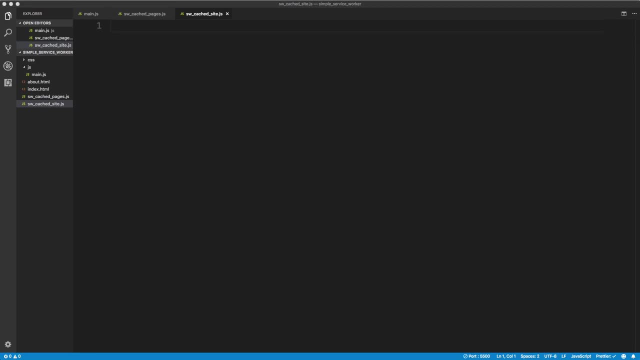 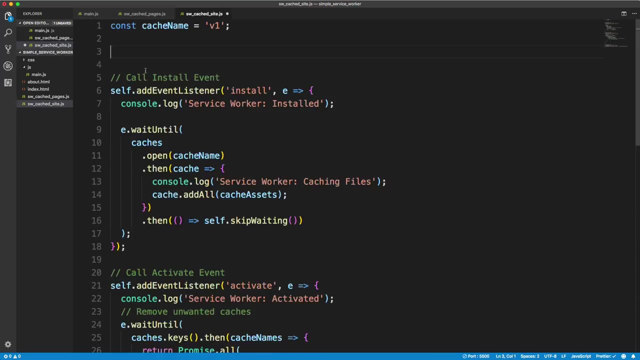 And I'm going to. Let's see how do I want to do this. Well, I guess we'll copy what we have here And paste that in, Except we don't need the cached assets. We do want to cash name. in fact, I'm going to call this V2.. 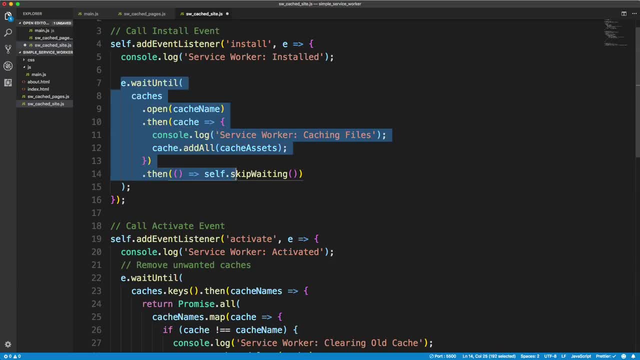 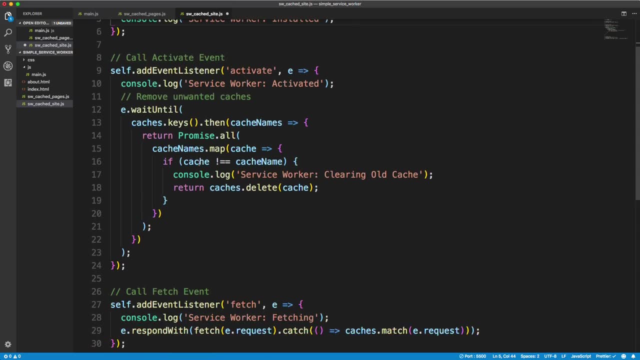 And then in the install: I'm not going to do the caching here, so I'm going to get rid of this, This, this wait until I'm still going to leave the event here like that, But not, I'm not going to do anything in it. 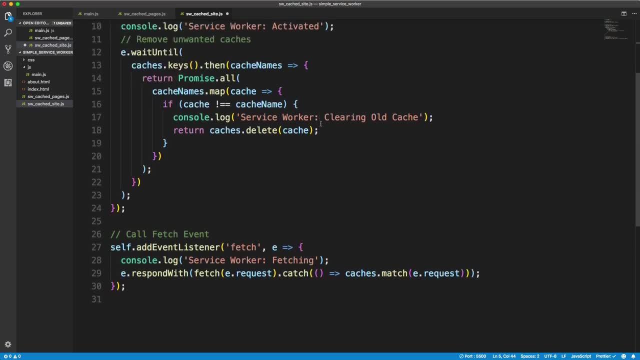 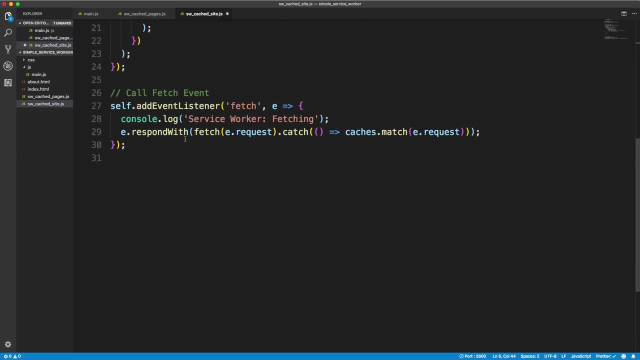 Activate is going to stay the same, because we still want to clear any old cache, But we want to do the real work down here in the fetch. OK, So we're going to have a respond with, just like we did before. Let's see. 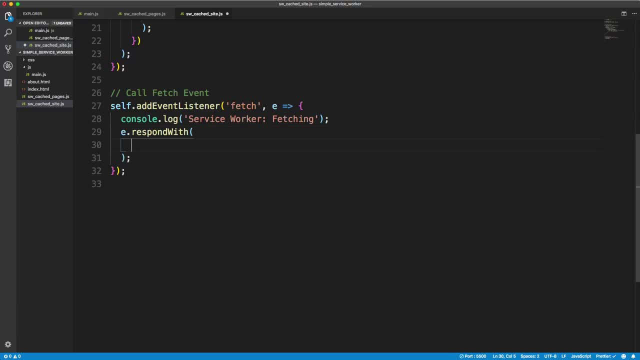 It's just clear this. so we'll say respond with, And then we want to fetch our initial request. so he dot request OK, And then that, Or Return a promise. so we'll do dot then, And then we'll get our response. 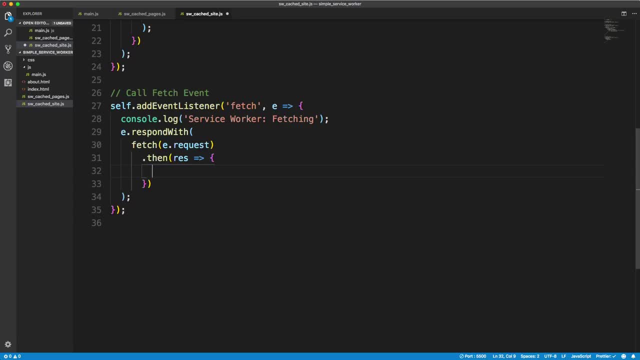 And then what we need to do here is basically make a copy of the response that we get from the server. So let's say, make copy or is actually a clone? so make copy clone of Response. and we can do that by creating a variable going to call it res clone. 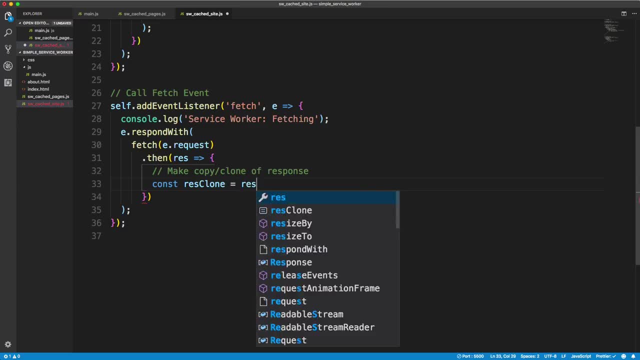 And I'm going to just set it to res and there's actually a method called clone. OK, So you want to set it to that? Then we want to open A cache, just like we did before in the install, except for doing it down here. 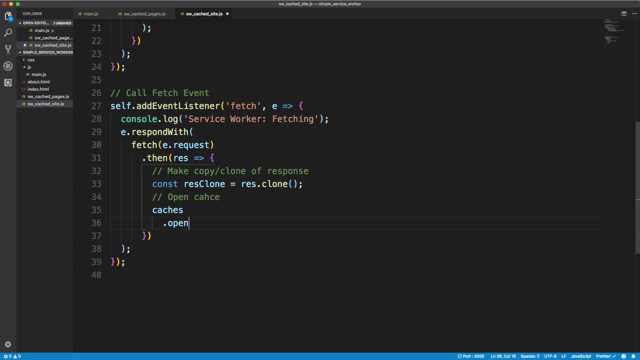 So we want to call dot open And we want to open Cash name which we defined above, And then that gives us a promise. So dot, then, And we get our cash object just like before. I'm going to set that, to set a curly braces. 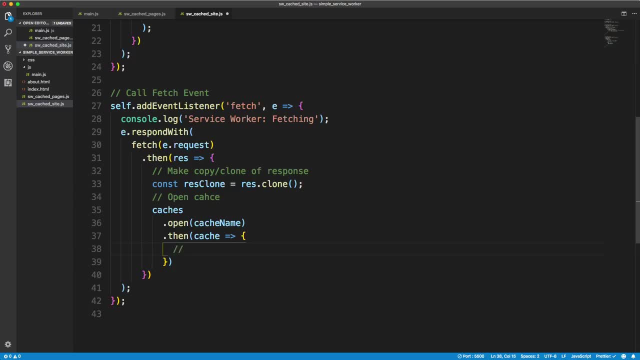 And Here we want to add The response to The cash. So we're going to say cash dot put. OK, So we use this put method. We take the initial response, which are the initial request, Which is he dot request. 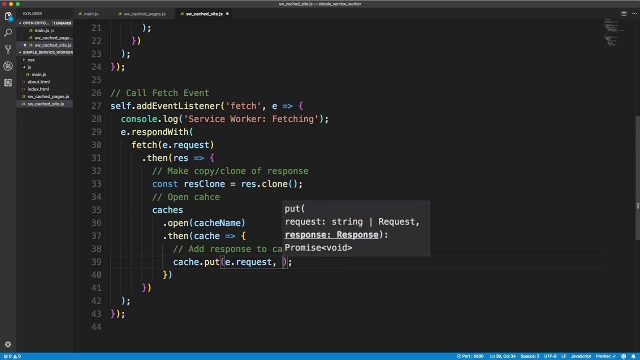 And then we want to put in res Clone, which is our copy that we made up here. OK, So res clone. And then we just want to return the original response. So down here, Let's see, we want to go under Right here and just return. 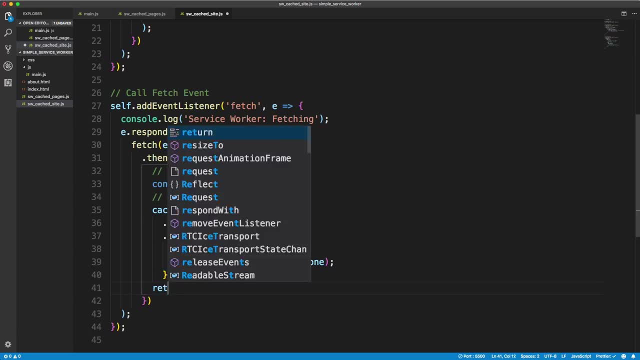 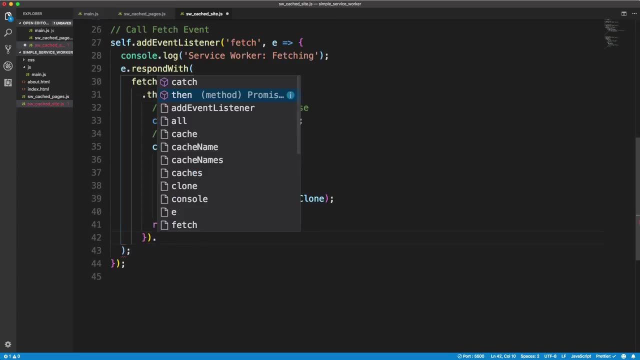 Res Like that. Now, if the connection drops, then This dot catch is going to run, And we should be able to see that, And we should be able to see that, And we should be able to see that. We should have our response inside. 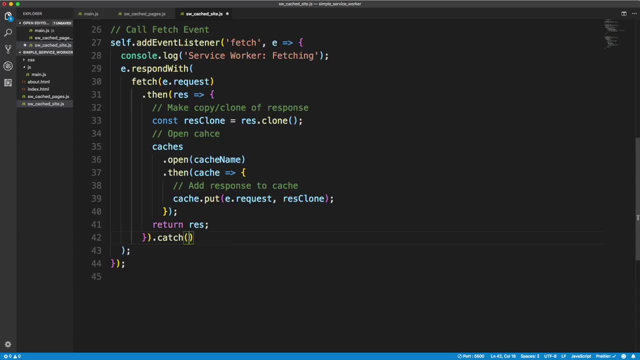 Of the cash right at this point. So what we can do Is: this will give us an error, And I'm just going to do an arrow function And we can say: Not catch Caches, Or yeah, Caches dot match. 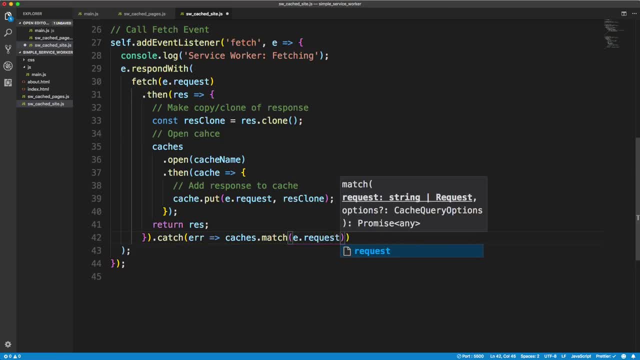 And we just want to put the e dot request, Because right now it should be in the cache. As long as the user went to the site once, Then it should be in the cache And This will have a dot then, Because this returns a promise. 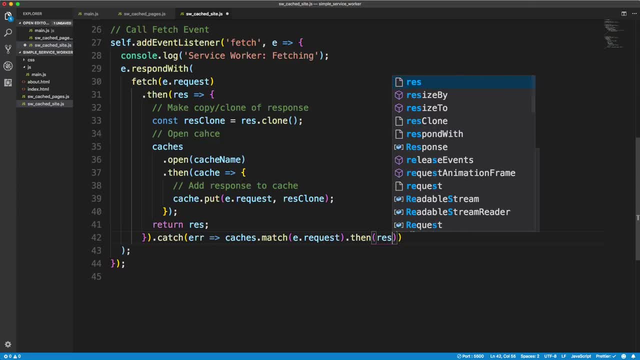 And we simply want to return The response, And since we're using arrow functions, We can just do it like that. If you're using regular callbacks, Then you just want to return res. But that should be good. Let's save this. 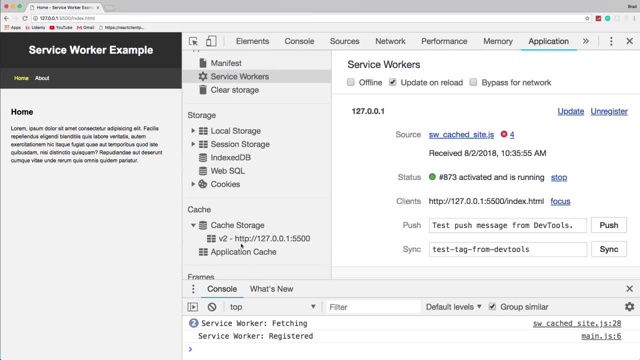 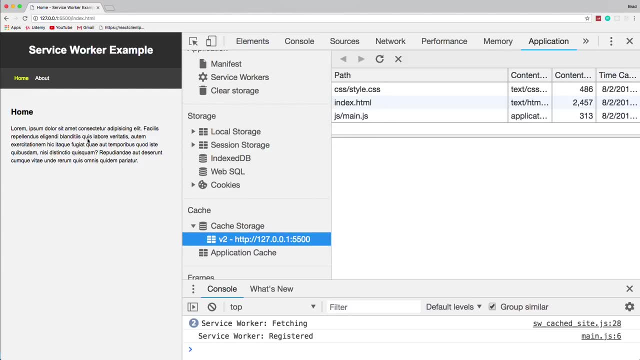 And now, if we go back to our browser And look in our cache storage, You'll see we have our index HTML that we're currently on, Plus the assets JavaScript that go with it. Now the about isn't here Because we haven't visited it yet. 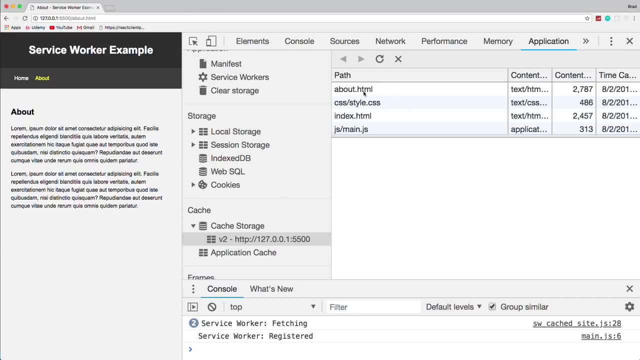 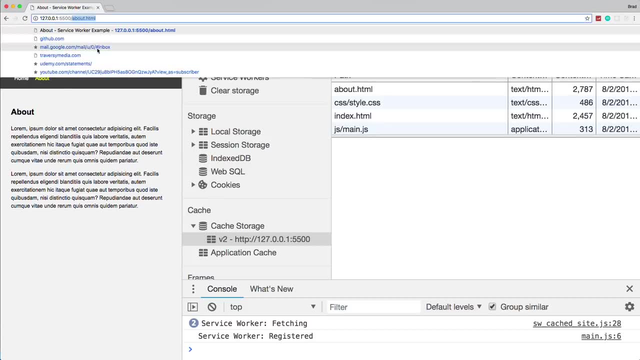 So if I click on about, That will automatically get pushed to cache. Okay, Because, remember, when we make the fetch- In this case we just made a request to, Or a fetch to the about- It's going to make a copy of it. 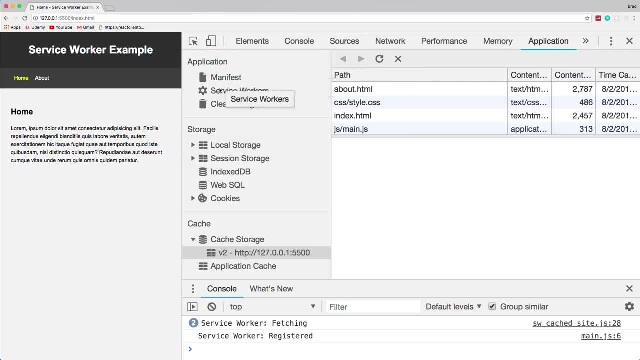 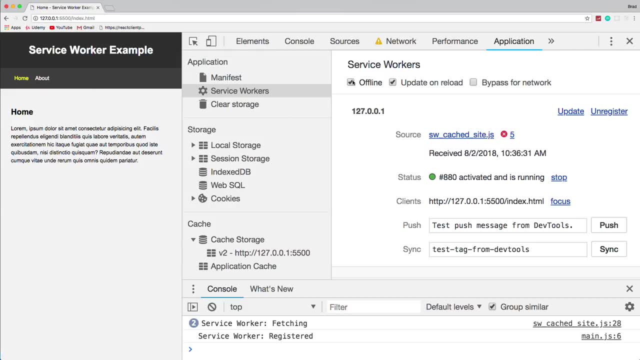 And put it into the cache, And now, whenever you're offline, You should still be able to access Those pages And those assets. Alright, So now what I want to do is test this out, So I'm going to push to github. 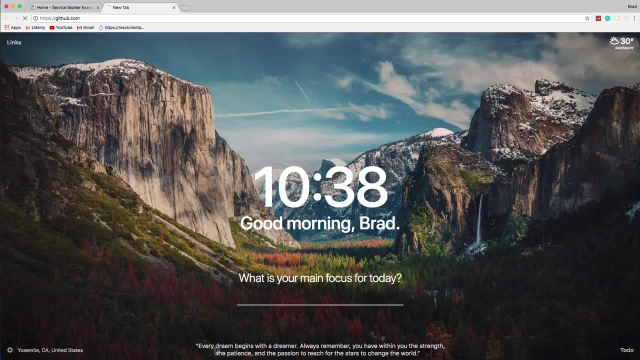 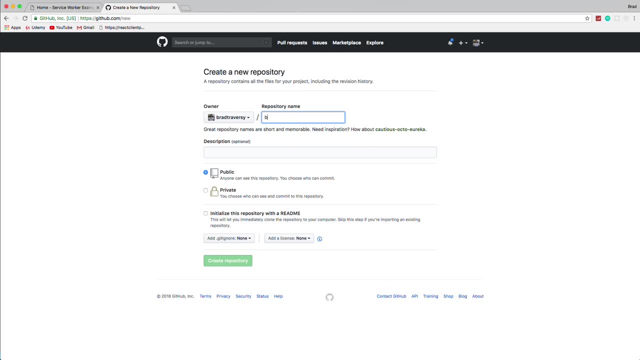 Okay, So we're going to use github pages. So let's go to githubcom, And the simplest way to use github pages Is just creating a repository With your username. So mine is bradtraversy, And then you want to do githubio. 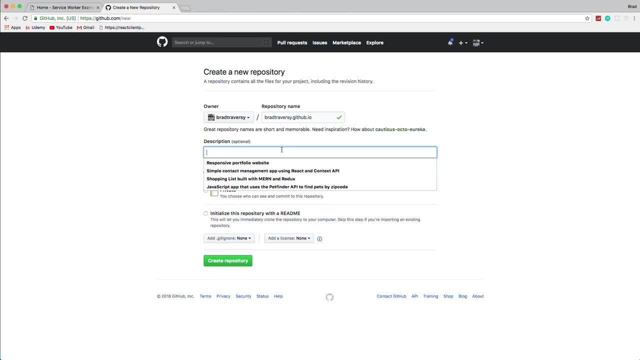 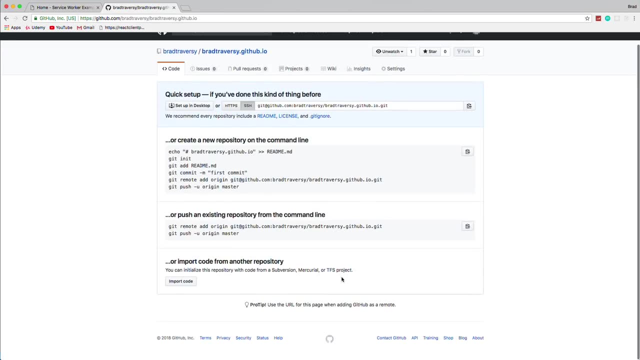 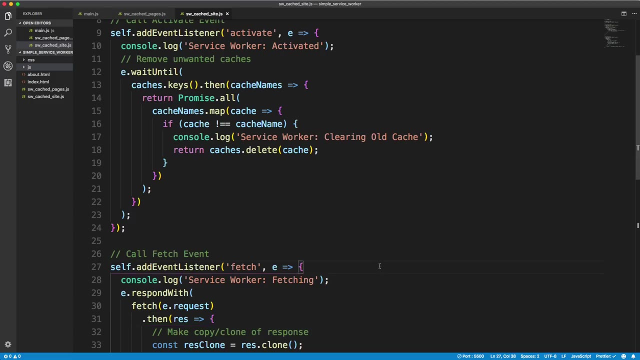 Like that And I'll just say: Test website And we'll create A repository. Okay, So now I'm not going to like go over The basics of git Or anything like that, I'm just going to push this to it. 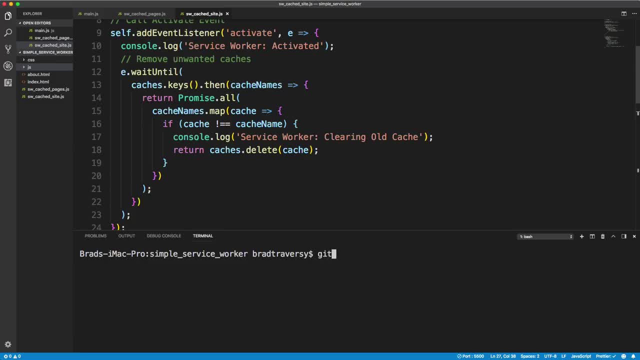 So we can test it out. So if you're learning about service workers, I'm guessing that you know git. So let's just git init And let's add all, And then we'll make a commit. Okay, So now that we did that, 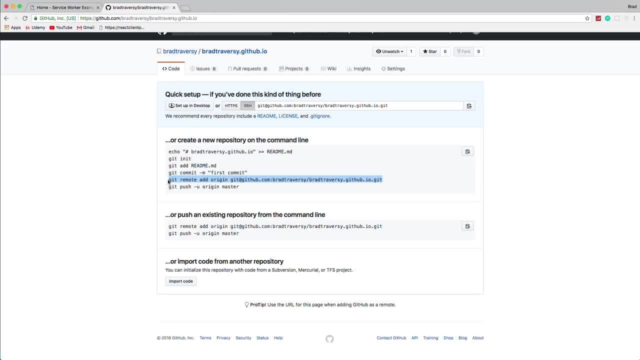 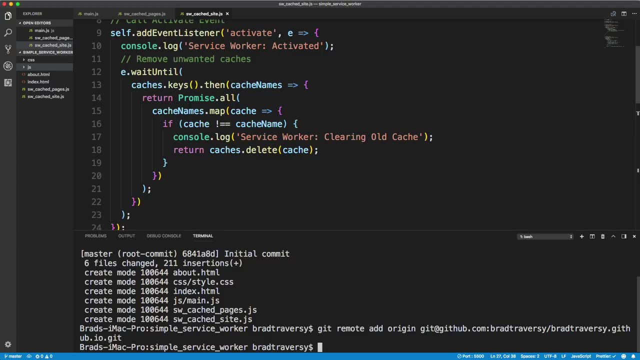 Let's add the remote repository, So I'm just going to copy this Right here And paste that in there. Sorry if you guys can hear that banging outside Doing construction. What else We want to do? our initial push, So we'll grab that. 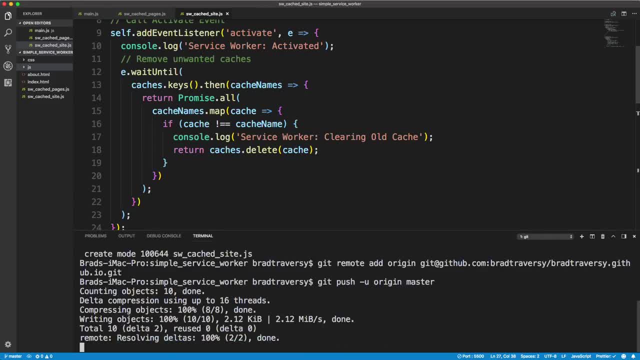 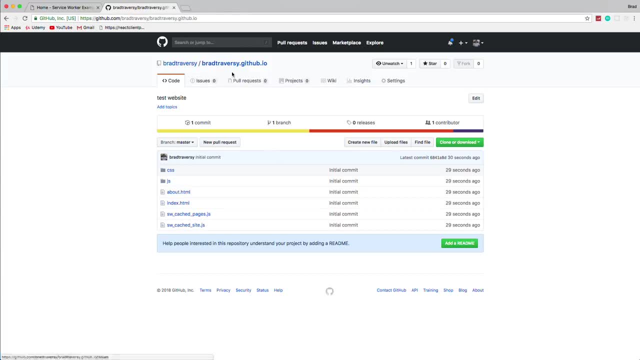 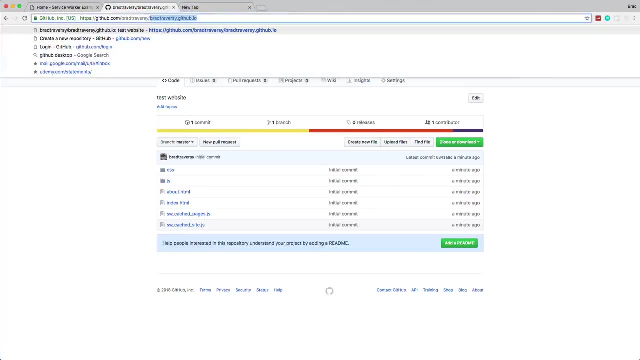 And let's push. Okay, Jesus. So if I reload this Now, we have our Repository here, So let's head to that actual Domain, Which is going to be bradtraversygithubio. And here's our website. 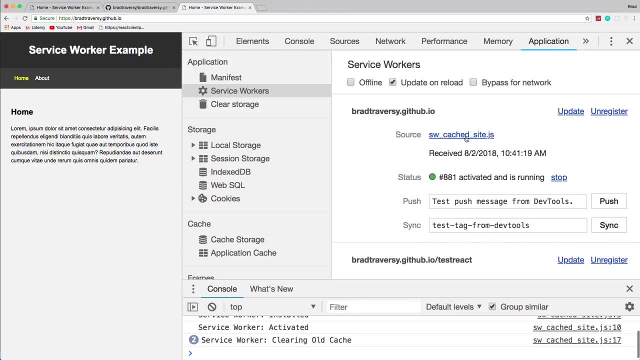 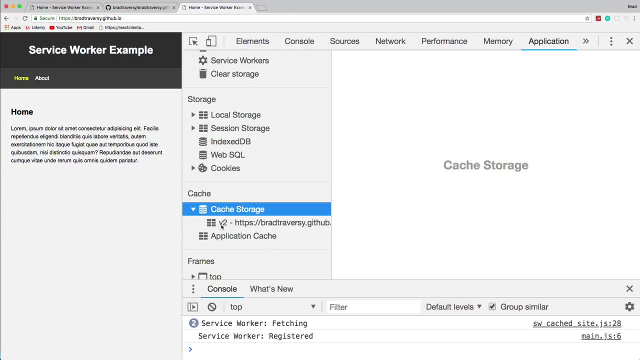 And let's open up chrome tools And you can see We have our cache site here. And if we look in, Let's see- I'm going to just reload this- And if we look in our cache storage, We have our index. 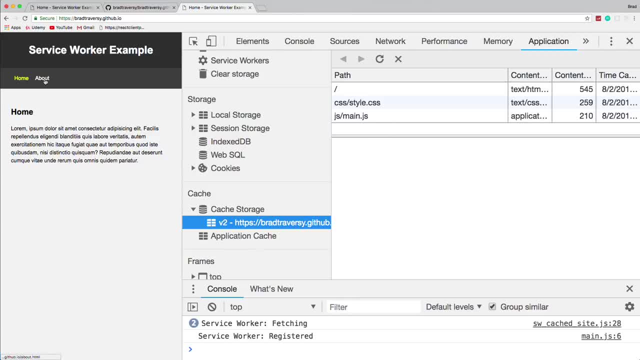 Which is slash. We have our css JavaScript. if I go to about That gets put in the cache. Now I'm actually going to test this By shutting off my internet connection. So I'm on a mac, I'm just going to go up. 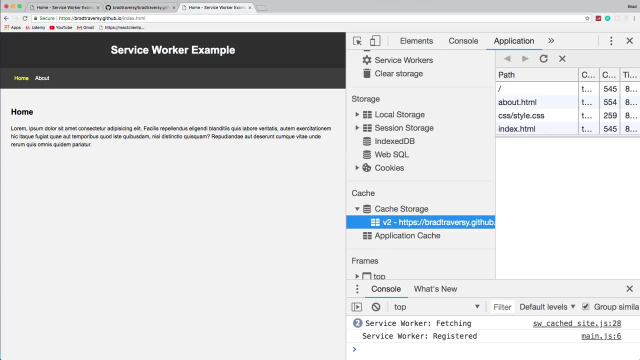 And this is connected through wifi. So I'm going to turn my wifi off And let's try it out. We'll reload And we still see the site Go to about. It's still there, Okay, And I'm going to prove to you. 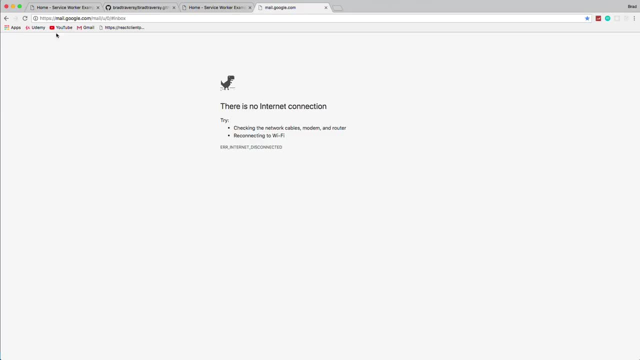 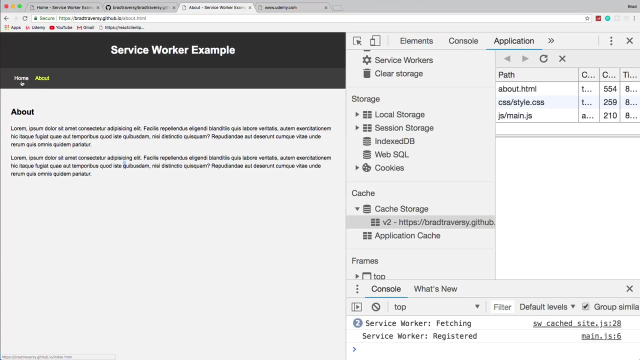 If I go to like, Let's go to youtube- No connection, Gmail- no connection, Udemy- no connection And our site works Alright. so this was a very basic tutorial And introduction to service workers. Like I said, There's libraries like workbox. 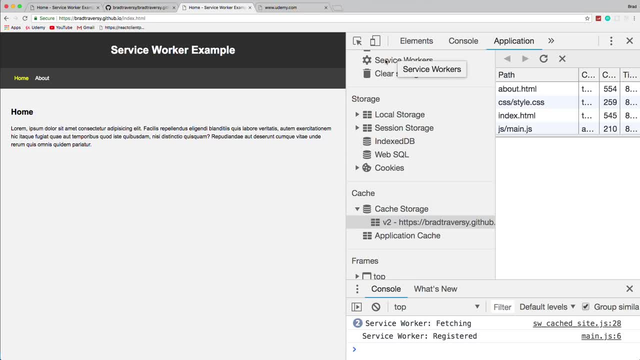 That make this stuff a little bit easier. But my goal was to give you a tutorial Basically on just vanilla service workers And just how to Call the install and activate Events and then fetch something And put it into the cache. That was the goal for this video. 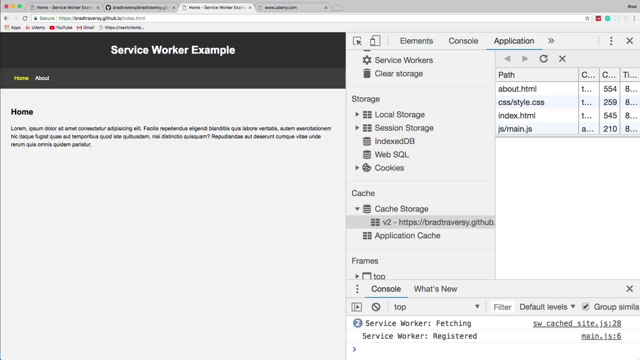 And I think we did that. So hopefully this helps you guys out. I will be doing more advanced stuff on service workers In the future, Including building a progressive web app With- probably with- react, Also thinking about doing one with view js.